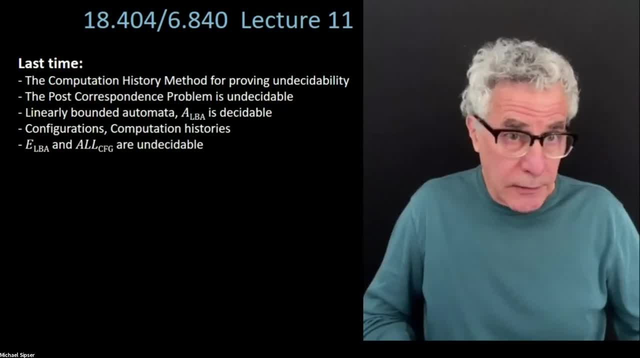 is given a Turing machine and an input, you construct a polynomial that has several variables And where the- in order to get an integer root, an integer solution of that polynomial, one of the variables is going to have to be assigned to some kind of encoding of a computation. 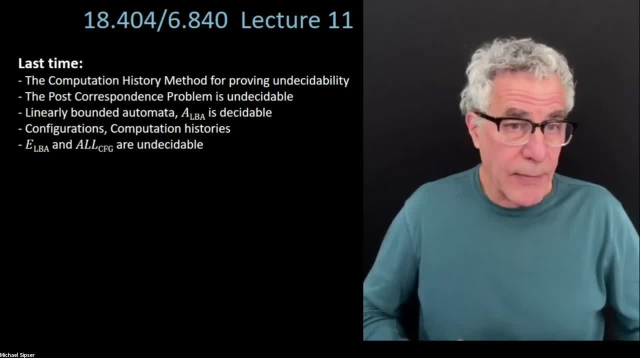 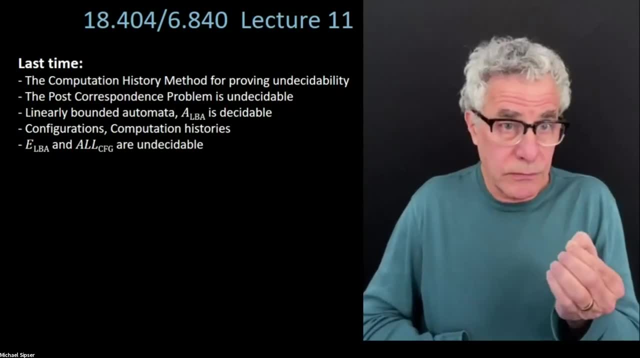 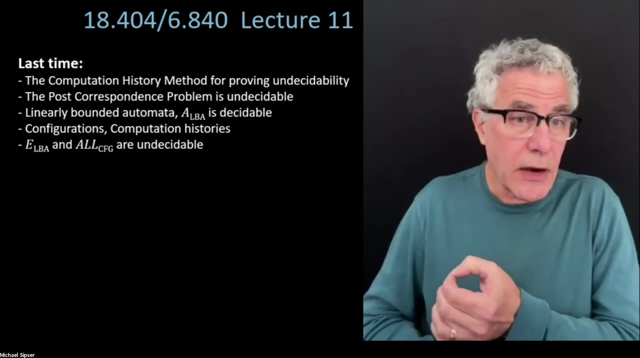 history of the Turing machine, of that of M on W. It's going to be. some one of those variables is going to be a computation history, an integer which represents the computation history for M on W, And the other variables are there to help you kind of decode that, so that the polynomial 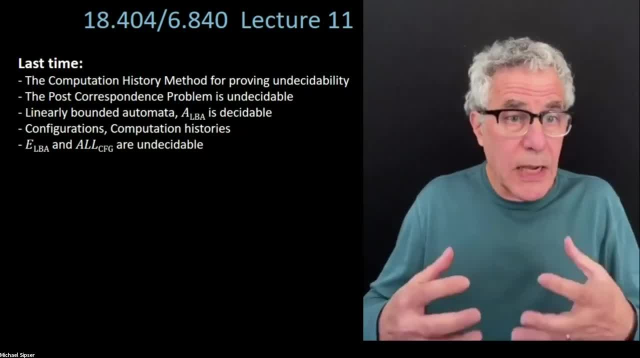 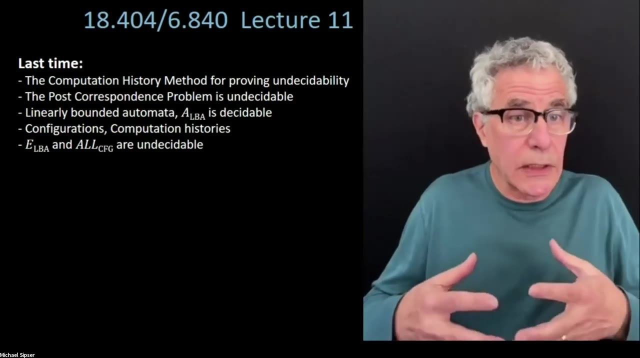 can actually check And make a solution. Yeah, A solution. It becomes a solution if that actually is a legitimate computation history of M on W. So it really uses the very same method that we've been using all along. But it's it, just it's. it's pretty hairy to construct that polynomial and do the check. 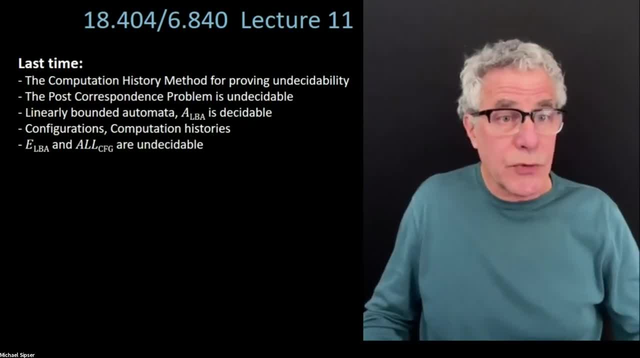 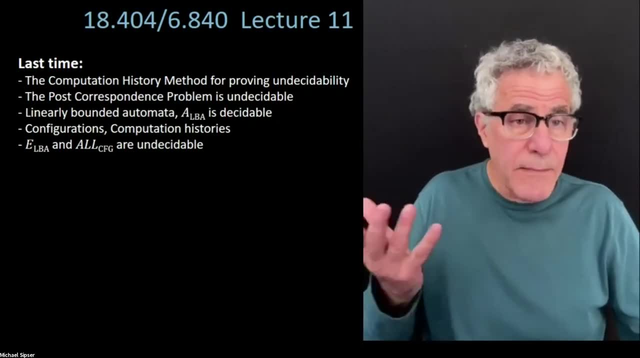 in the way that you need to do So. for the post correspondence problem which we introduced last time it's doing the check is relatively simple. You know that the, the match is the, is the computation history And you know following the rules of the match is fairly simple to construct that post. 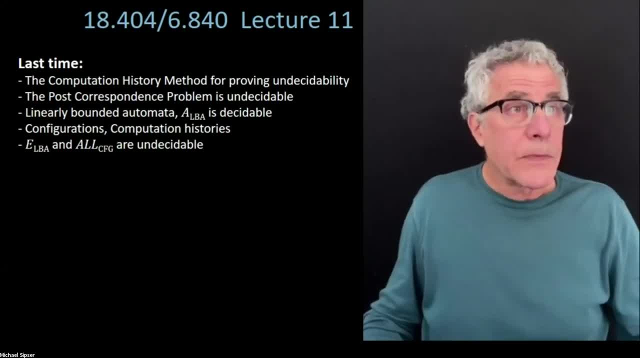 correspondence problem instance. We talked about linearly bounded automata. You know, we, of course we defined configurations and computation histories along the way, and proofs are on a certain problem. Other problems are undecidable as well using the same method. Okay. 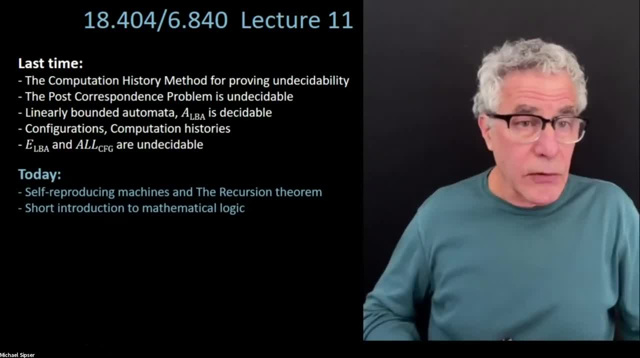 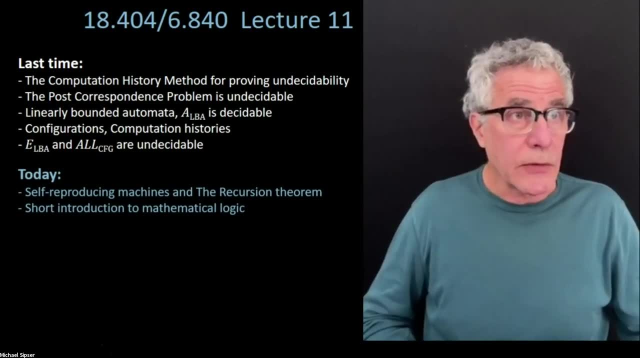 So today we're going to shift gears. We're going to, In our last lecture on the computability section of the course, we're going to talk about something called the recursion theorem, which basically gives Turing machines the ability to refer to themselves Turing. 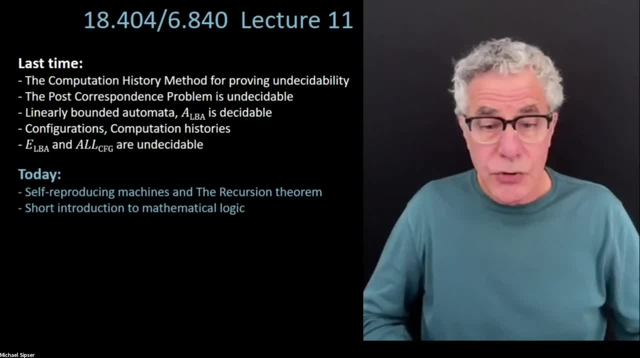 machines in any program to do self-reference, so that you can actually get at the code of the Turing machine or the code of the program that you're writing, even if that's not a built-in primitive of the programming language or the operating system that you're working with. 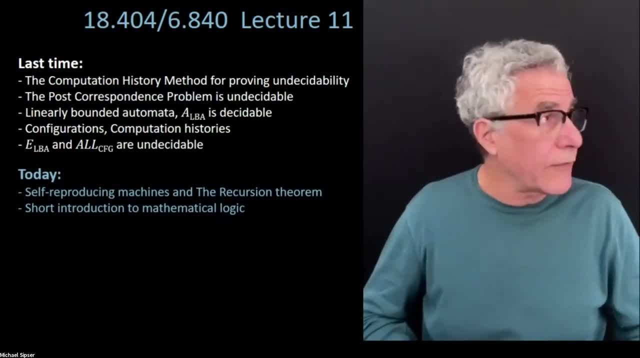 It still gives you that access. And also, if we have time, at the end, I'm going to talk a little bit about mathematical logic, which is sort of a nice application of the recursion theorem, And it's a beautiful subject on its own. 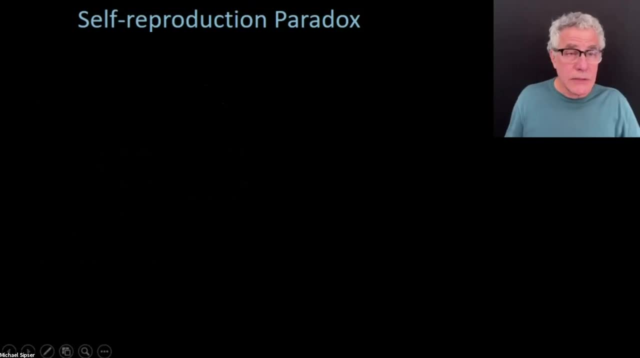 and it's something that I can give a brief introduction to. OK, so today's topic is about self-reference, self-reference, Self-reproducing machines and the broader topic called the recursion theorem. So let me introduce it with what I would call the self-reproduction. 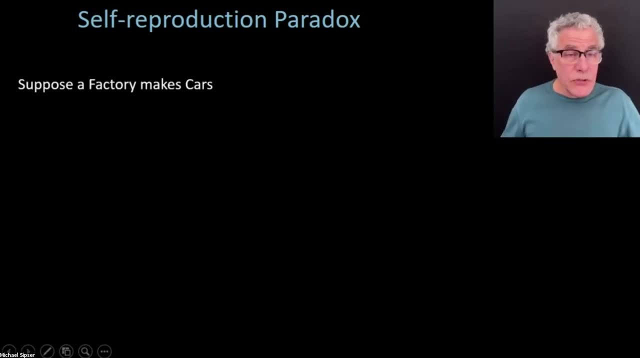 paradox, And that is suppose. you have a factory like a Tesla factory, a car manufacturing factory. Here's a picture of the factory and it's producing cars. All right, So we have a factory that makes cars, And what can we say about the relative complexity of the cars? 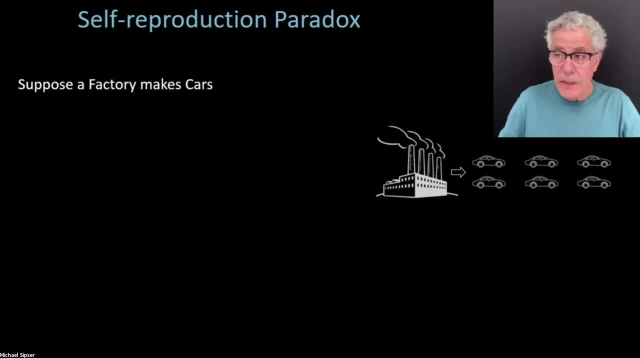 compared with the factory in some informal sense. So I would argue that you would be reasonable to say that the complexity of the factory is going to have to be greater than the complexity of the car And the complexity of the cars that it makes, Because not only does the factory have 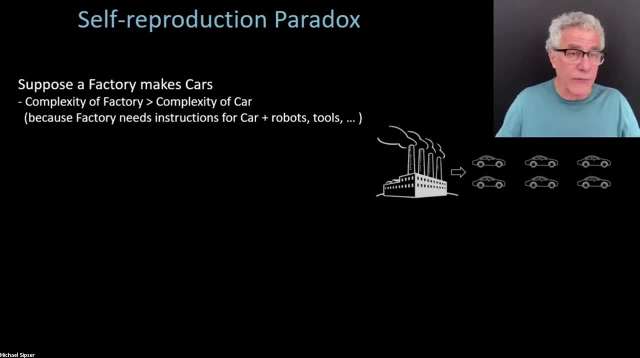 to know how to make the cars, so it has to have all the instructions and whatever things that go into a car. it has to be included in the, at least in some kind of. it has to be in some sense represented in the factory. 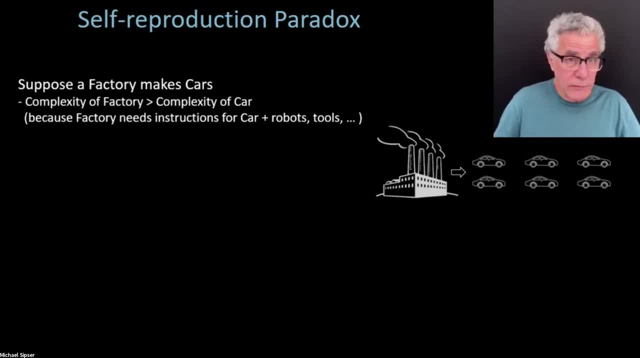 But the factory also has to have other stuff: the robots and the machine And the other manufacturing items, tools and so on for making the cars. So the factory has to have all the complexity of a car incorporated, plus other things as well. 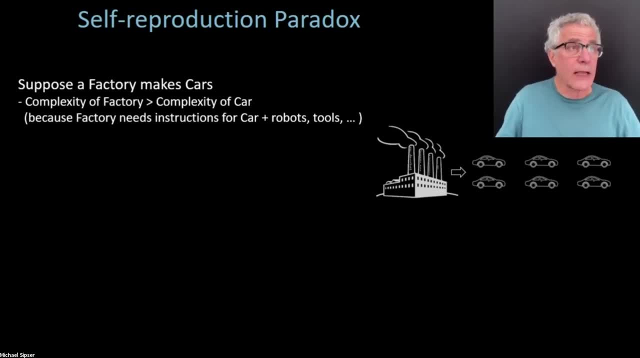 And for that reason one could imagine that the factory's complexity is more than the car's complexity. But now suppose you want to have a factory that makes factories, So imagine, here's the picture. So, or in general, a machine that makes copies of itself. 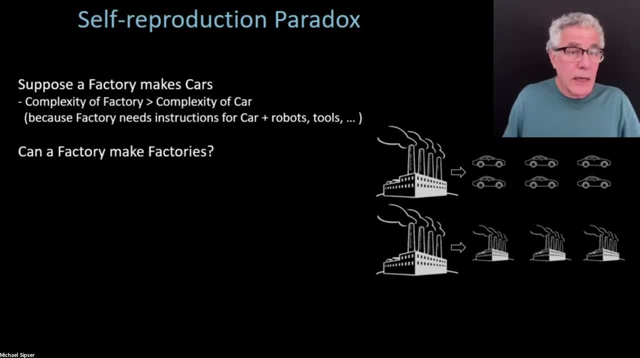 Well, that seems at first glance to be impossible, Because not only does the factory obviously have to have all of the instructions for what a factory is like, but it needs to have all of the extra things that it would need to do the manufacturing. 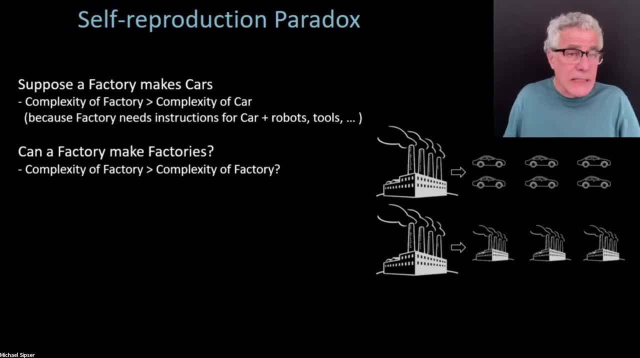 And so for that reason It seems like a. it's not possible to have a machine make copies of itself. I mean, you would run into the very same problem if I asked you to produce a program in your favorite language that prints out itself an exact copy of the same code. 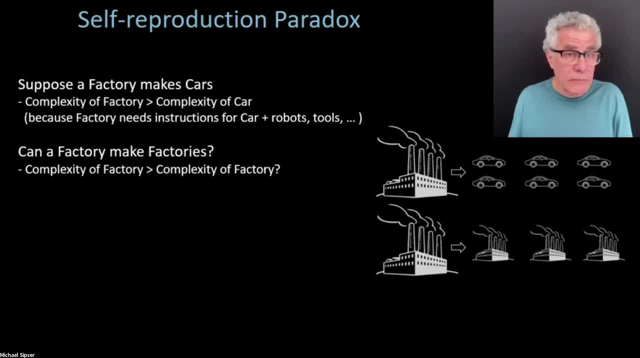 I mean you can always write a program which is going to print out some string you know, like hello world. That's easy you, because you just put hello world into some kind of a variable or some sort of a table into the program. 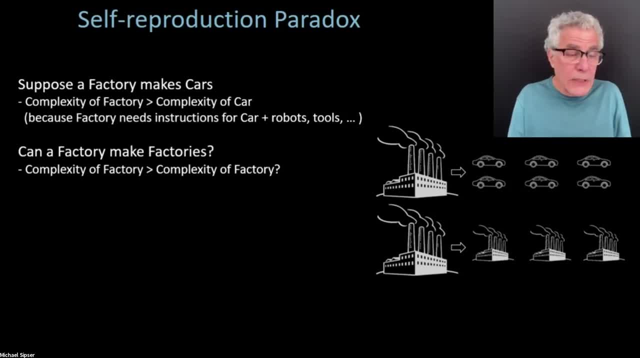 and say: print that table. But if you want to make a print of, if you want the program to print out a copy of itself, you can't take the whole program and stick it into a table because you know the program's going to have to be bigger than the table. 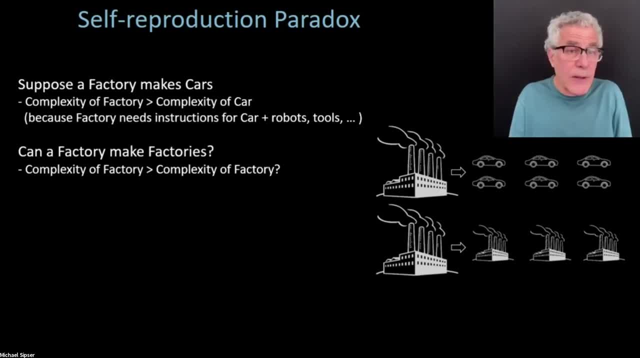 You know, And so you're going to end up with something that isn't really that big. impossible will happen, because the program, an entire copy of the program, can't fit inside the program. You just get the program inside itself, inside itself, inside itself forever, And so you. 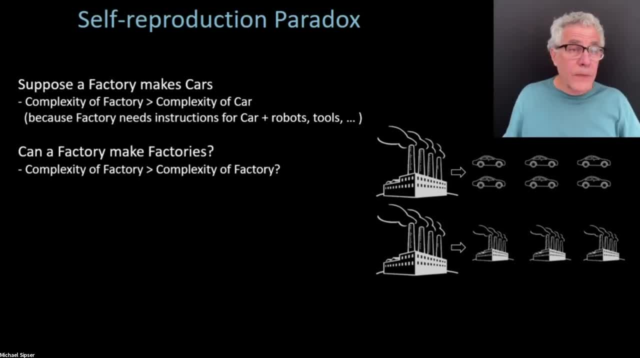 end up with like an infinite program that way. So if you just kind of naively approach the problem for how to make a program which is going to print out a copy of itself, it's not so easy to do But hopefully after today's lecture you'll see that it is possible and in fact how to do it. 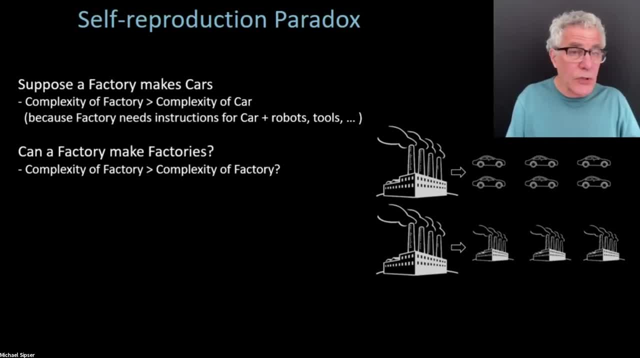 And not only that is an idle bit of curiosity, but there are actually applications for why you might want to do that, mainly within mathematics and in computer science theory, But there's even a kind of a real world application, if you will, in a way too. So we'll get to that at the 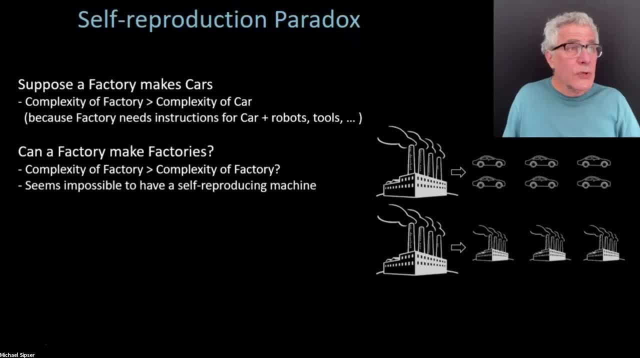 end. So it seems, as I'm saying, impossible to have a self-reproducing machine, But we know that in the world there are things that make copies of themselves- living things. So it seems like a paradox. You know, cells can make copies exactly of themselves. All living things can make copies. 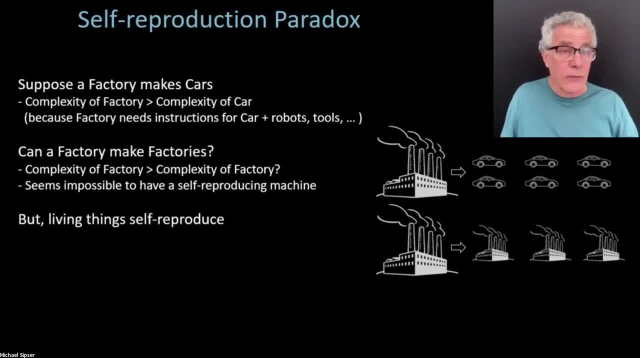 of themselves. So how do they manage to get around this paradox? Well, in fact, there's no paradox, because it is possible to make a machine that self-reproduces, that makes copies of itself, And this has been known for, you know, for many years. Probably it goes back. 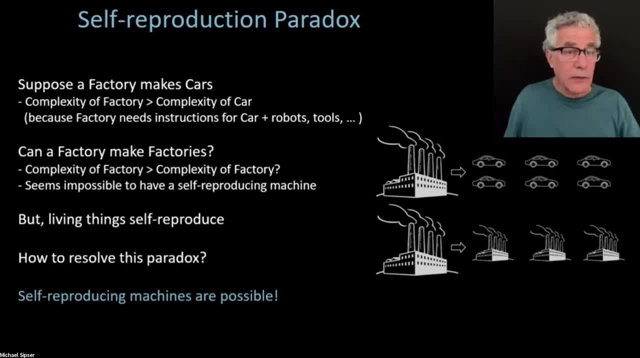 to von Neumann, who wrote a famous paper on self-reproducing machines. Okay so, self-reproducing machines are in fact possible. So let me give you an example of how you would make a self-reproducing machine. 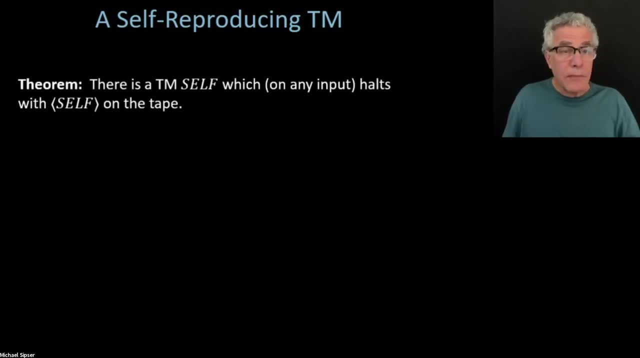 Turing machine. What do I mean by that? I mean a machine- I'm going to call it self- which ignores its input. So on any input you turn it on, the machine grinds around for a while and holds with a description of itself. on the tape, with a description of self, its own code. 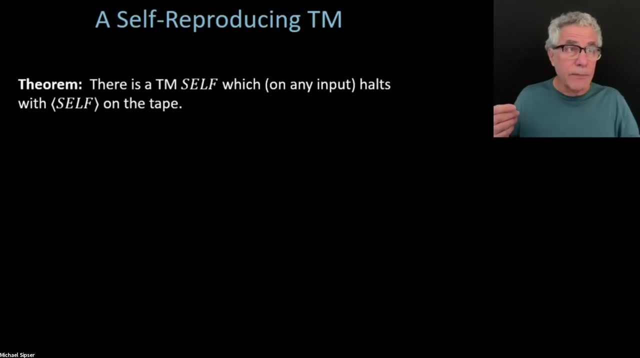 sitting on the tape, So very much like producing a program which would print out its own code. That's really what we're doing. So for that we're going to first need a little lemma, which is a very simple lemma, but it looks worse than it is, So let me just read it out. 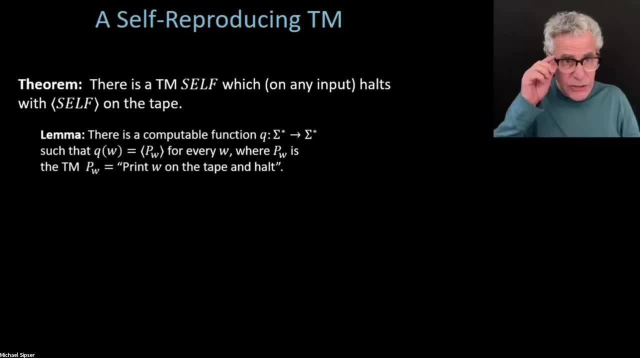 to you and then I'll explain what it's saying, because what it's saying is extremely simple. So there's a computable function- I'm going to call it Q- that maps strings to strings, which will will take any string, W, and produce from W a Turing machine which will print W. 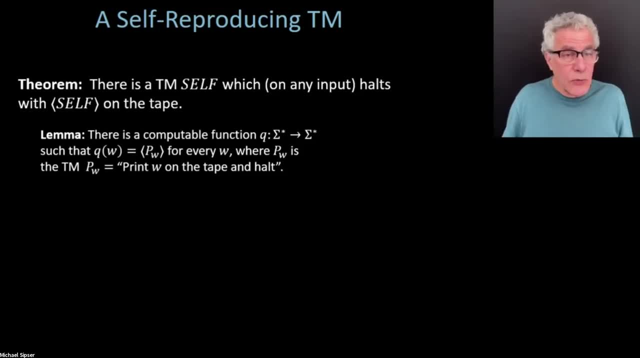 Okay, that's all it does. So, as you know, if I give you a string W, you could produce a Turing machine which would have W represented in the states and transitions of the machine, so that if you turn the machine on, the machine will be will output W. I mean, if I want you to. 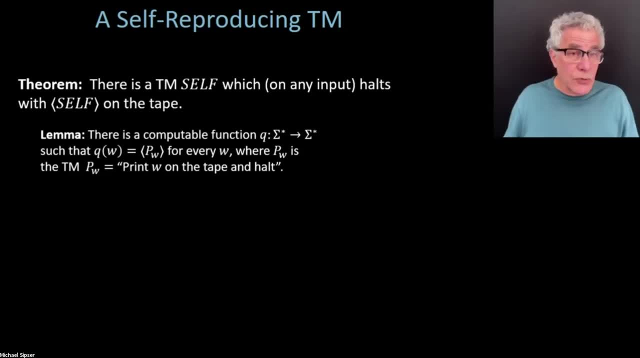 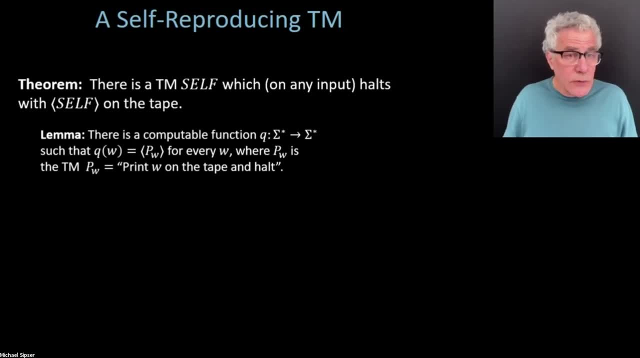 Um, and I'm, and if, no matter what the string was, instead of 1100 or one, you know whatever it's- you know 20 zeros and then five ones. you could do that too, And, in fact, um, there's a. 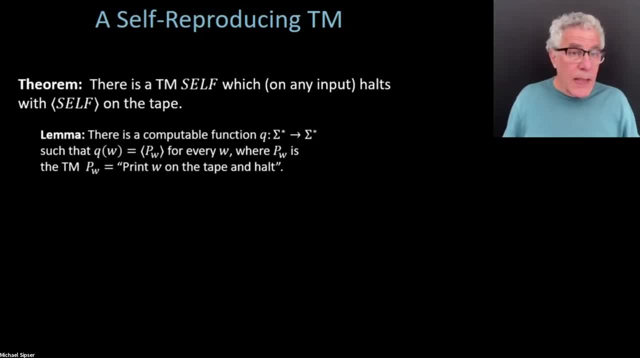 simple, simple procedure that takes a string and maps that onto a Turing machine which prints out that string. So that's a computable function which basically takes a string and converts it to something that evaluates to that string, And I'm calling it Q. I don't know if this 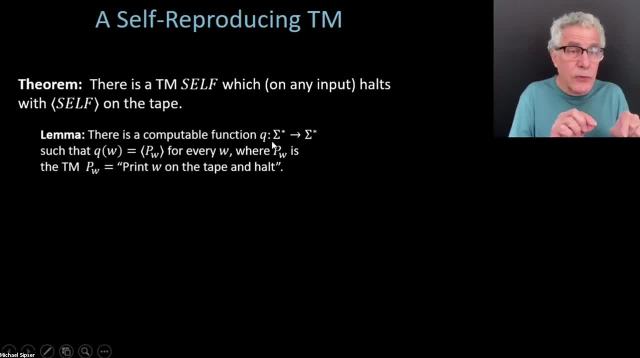 is helpful to you or not. It's kind of like it converts the string W to W in quotes, So Q stands for quotes in a way. So if that's helpful, then good. But anyway, P sub W is a Turing machine. 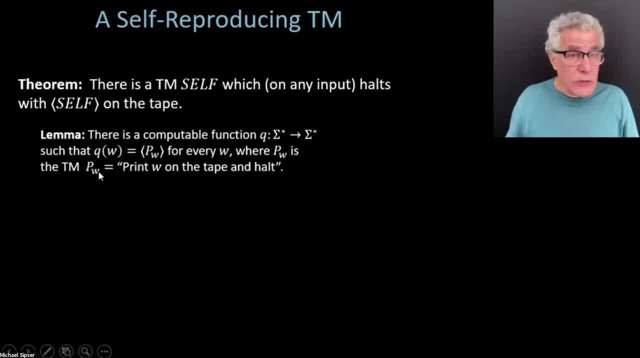 When you turn it on, it just prints out W and holds. And I can find P sub W from W, Straightforward proof. So now I'm going to tell you, assuming that we have that computable function, function Q, I'm going to tell you: 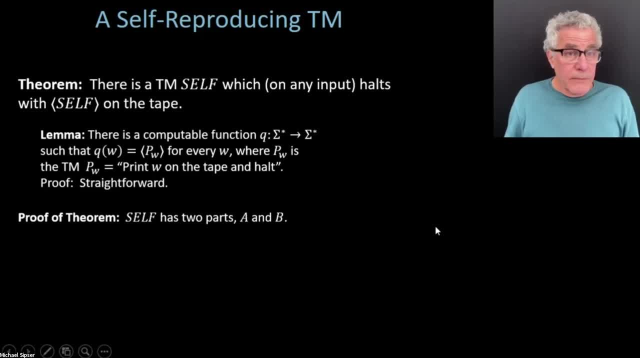 how to make this machine self And it's not complicated. The Turing machine self is going to have two parts, I'll call A and B. Here's a schematic for the machine. So here's self. It's in two parts, A and B. And what I mean by A and B. 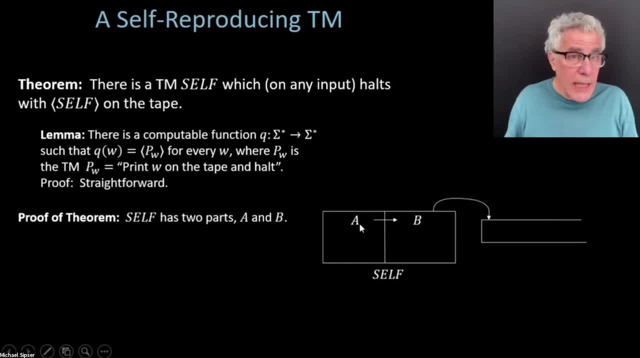 it's like two subroutines: Self, It's going to start out running A And then, when A is finished, it's going to pass control to B, And then B is going to finish the job And when it's done, you're going to have the description. self. 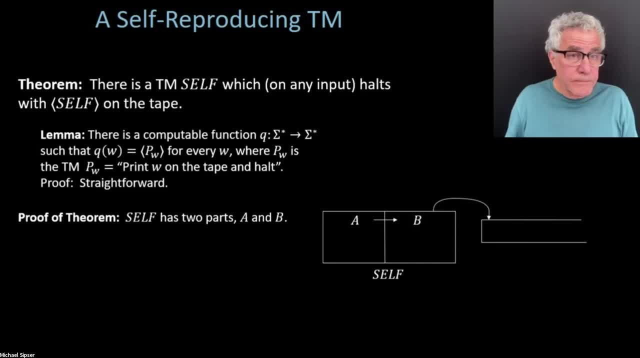 sitting here on the table. All right, So what's left is to give you the code for A and for B. So A is going to be something super simple. A is going to be that machine which prints out B, prints out a description of B, the one. 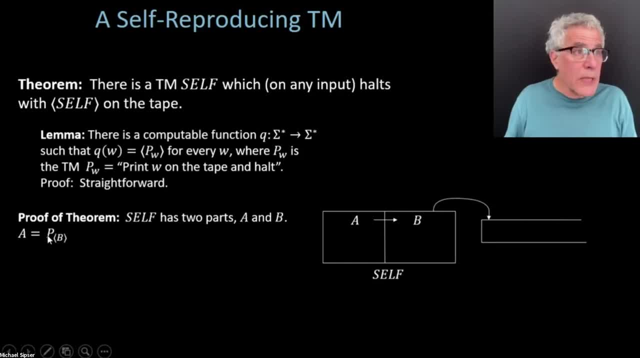 that I described up here. So remember: P sub W is the machine which prints out W And P sub. the description of B is simply going to be a machine that has this string P sub B stored in its states and transitions. You turn on that machine and it prints out B. 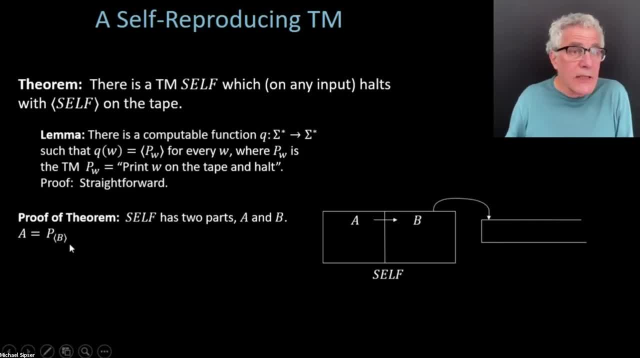 And then it's done. So this is a very simple machine. It's going to be a machine that prints out B, And then it's done. So this is a very simple machine. A is very simple, So here just to hear P sub B is a part of A. 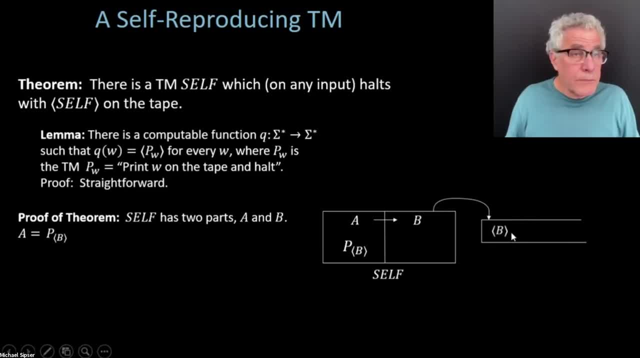 And when it's done, B appears on the tape. So that's at the point when A has finished its work. Now it's going to pass control to B. So we're not obviously done yet, because what we want is A and B both to be on the tape, not just B. 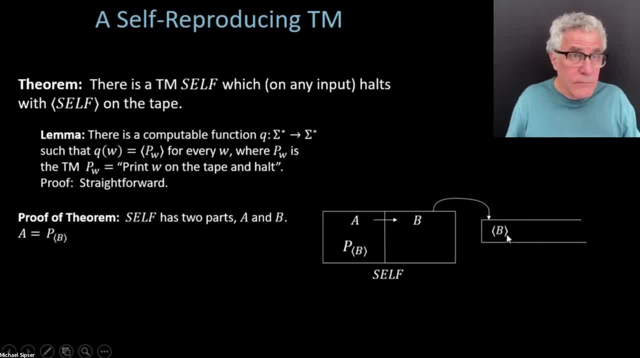 Because self is a combination of A and B together. So I have to tell you how B works to finish the job. So you might think as a first, given what we did for getting B on the tape, that we'll get A on the tape in the same way. 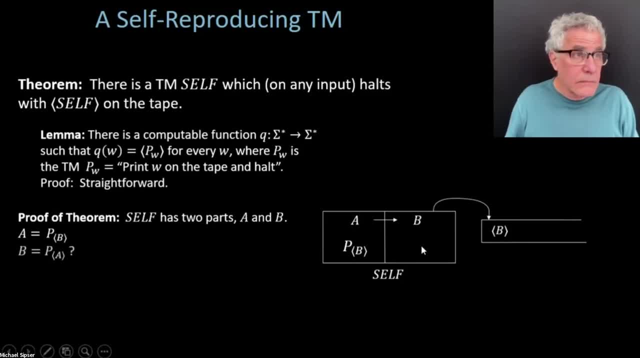 by putting a copy of A inside B, So a copy of B can be printed by A inside B, So a copy of B will come in. It won't work, It doesn't work, It doesn't work, It doesn't work. 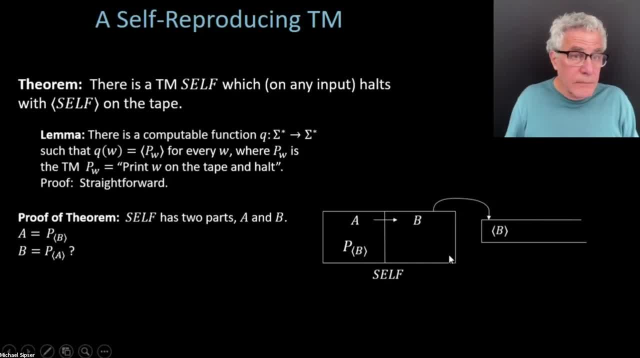 inside A and a copy of A is inside B And at some conceptual level that seems like that might do the job. but that is not a solution, Because the fact that I can put B inside A kind of forbids me from also putting A inside B, because that's going to be the same kind of circular reasoning. 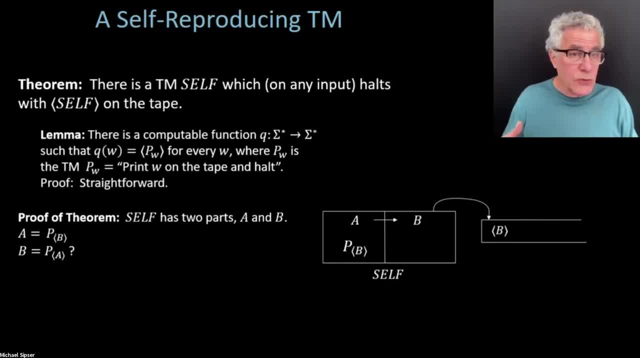 of just putting a machine inside itself. You just can't do that because you're going to end up with an infinitely big machine that way. In fact, if I'm putting B inside A, a copy of B in terms of its description inside A, A is really going to be much bigger than B, because it has all of B. 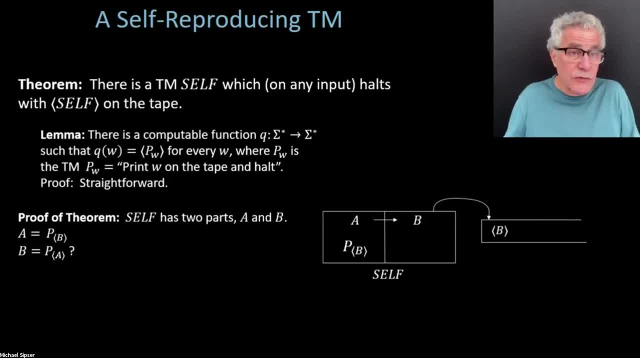 inside it, plus other stuff, all the states and transitions for printing that B out. So I can't have A be much bigger than B and then B also much bigger than A, So something this is no good, But we can do it. 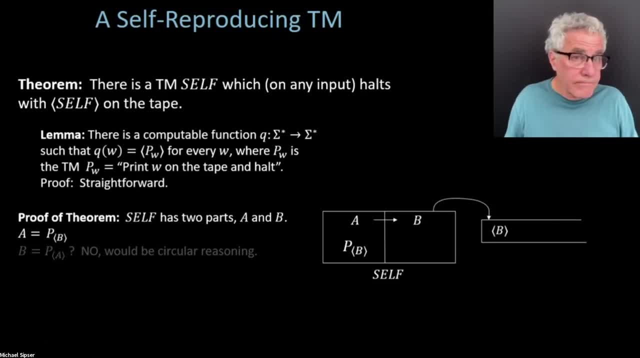 But we can do it. We're going to have to do something else. So how is B now going to get a hold of A? And the trick for doing that without having a copy of A inside B, which doesn't work. that's not going to be a good solution Instead of the way that B is going to get A. 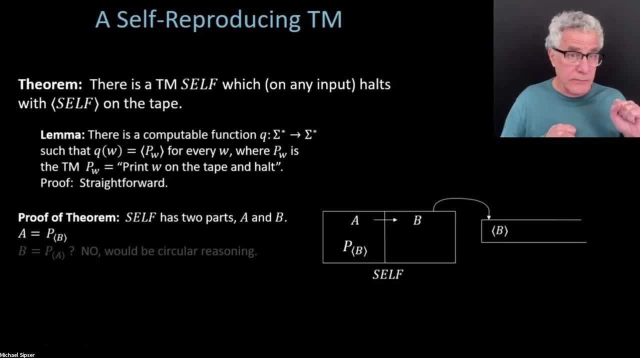 it's going to figure out what A is. It's going to figure out. It's going to figure out what A is. And how is it going to figure out what A is? Because if you remember B can look at the tape. It sees some string there. 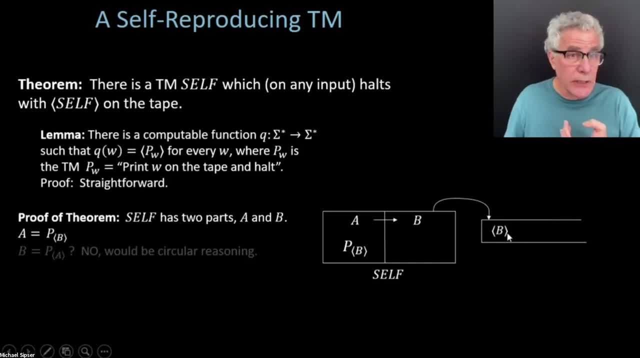 which happens to be a description of itself. but it doesn't care. It sees some string on the tape. A is the machine that prints out that string A is Q of this string. So B is simply going to compute Q of whatever it sees on the tape. 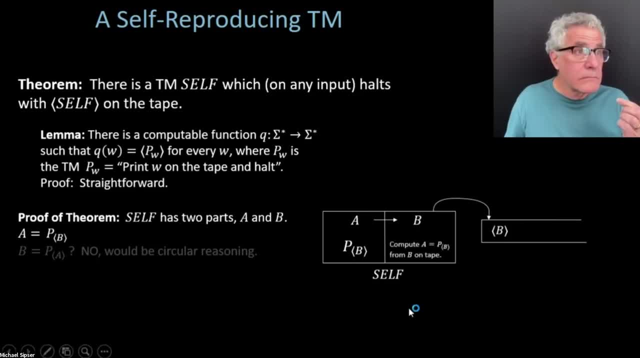 That is A. OK, So it's. I don't know if you can read this kind of small here. It's going to compute A from B sitting on the tape, So here is the instructions for B. It's going to compute Q of the tape contents, which happens to be. 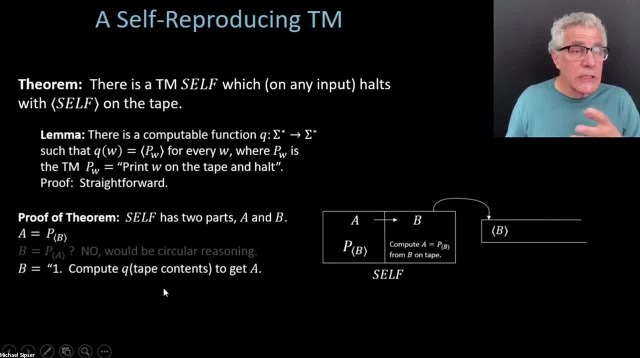 the description of B, but that's irrelevant to B. B just sees some string on the tape. It computes Q of that and that is the. that is A, Because A is the machine which prints out that string. Then it's going to combine A with B, doing whatever you know. 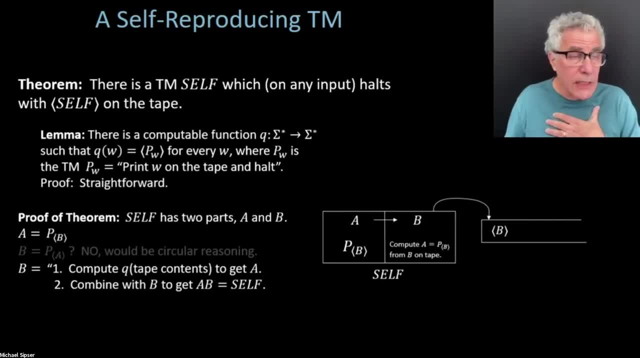 slight interfacing that needs to happen- I'm not going to get into those details- to convert those two pieces into one machine, which is the machine itself, And then it's going to print out with self on the tape, as I'm going to indicate over here. 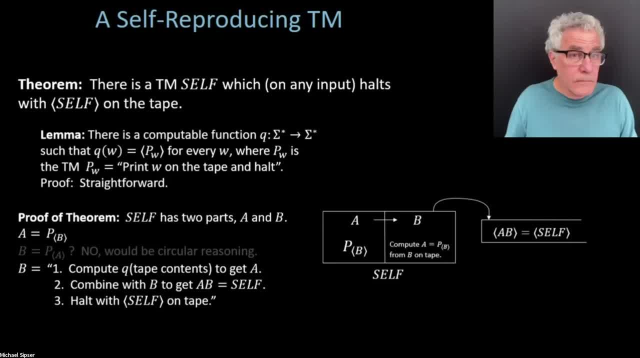 OK, So that's how a Turing machine can print out a copy of its own description and leave it on the tape. So, and what's nice about this is nothing specific about Turing machines, This is a general procedure, OK, That allows any programming language to print out a copy of its own code. 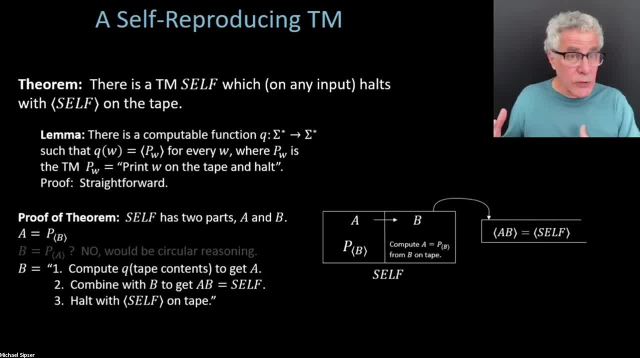 You can even carry this out in English, as I'm going to do in the next slide. OK, So here's a good question. There are many possible Turing machines that can print out B. That's right. How do I know? how do we get the particular one? 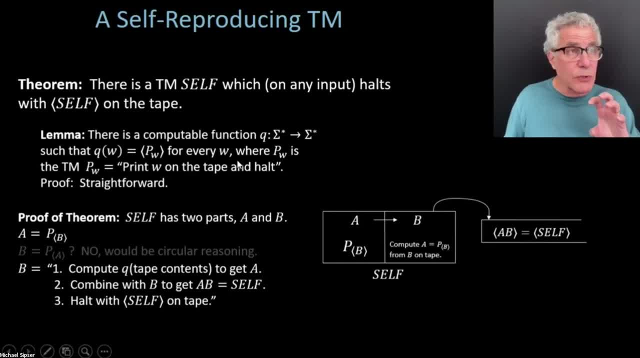 What I have in mind. that's a little bit of a subtle question, but it's a good question. I have in mind the particular Turing machine that prints out B, which is the one that Q produces, Remember so we. you have to refer back to this lemma. 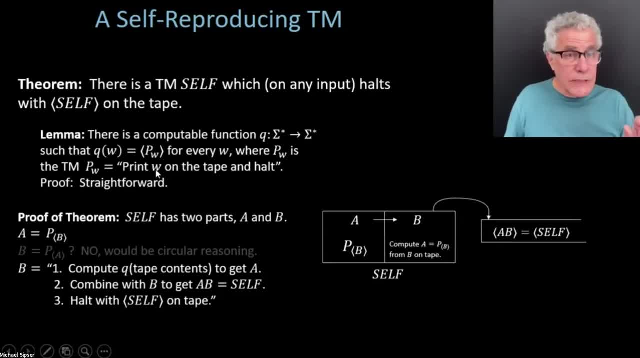 This lemma produces a particular machine that prints out B from B And that's the one that I'm going to use for A And that's the one that B is going to be able to obtain by running the Q algorithm to figure out B. 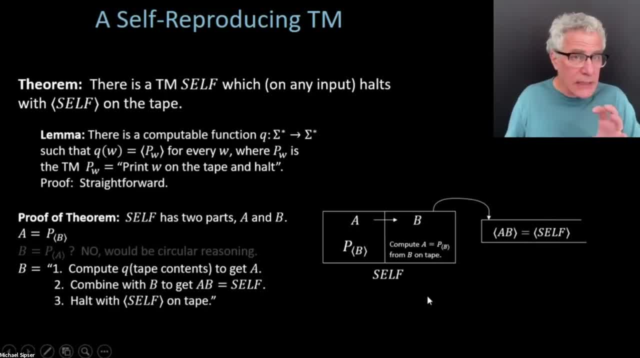 To figure out what A is. So you have to make sure you're being consistent, And that's a little bit of a detail, but it's a good question. Why doesn't this create a circular argument too? Well, there is no, so that was another question I'm seeing here on the tape. 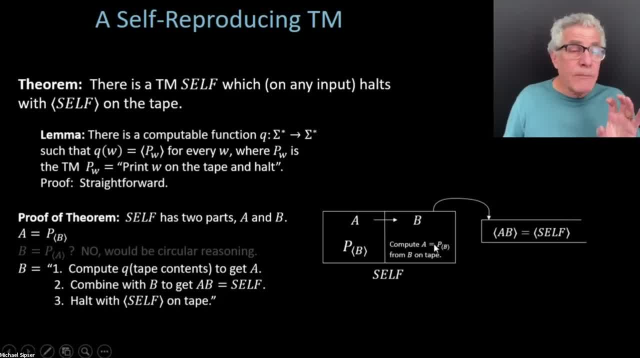 Well, there's no longer anything. See, B does not have to have A stored within it. It figures out A. So in a sense, you're going to write the program, the code for B, first. B is just a simple program. 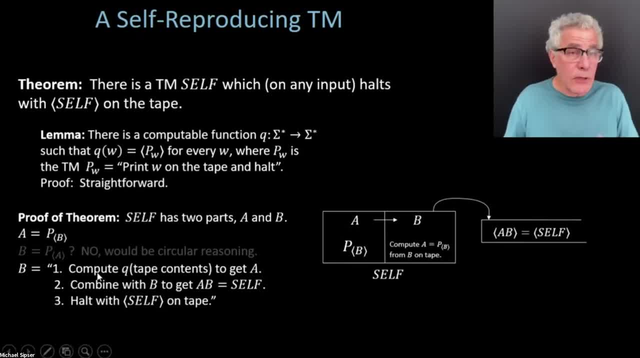 Here it is. There's nothing circular about it. It says B is a simple. the code for B is: take a look at the tape, compute Q of that, combine the result with whatever was sitting on the tape from before and print it out. 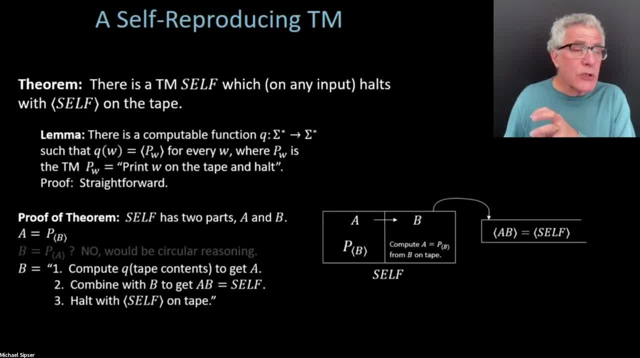 I mean that's a piece of code which you can just write. I mean this will become more clear, hopefully, in our next slide where we talk about the English implementation. But just, I don't want to rush to that, So you can figure out B without even knowing what A is. 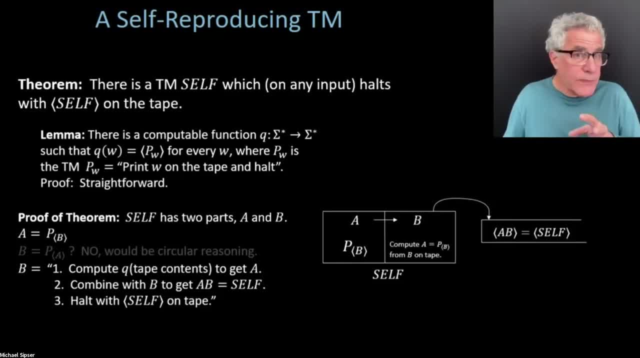 B stands alone, But then because B is just a piece of code that runs Q based on what it sees on the tape A. now you need to know what B is in order to obtain A, Because A has the code for B embedded within A as a string. 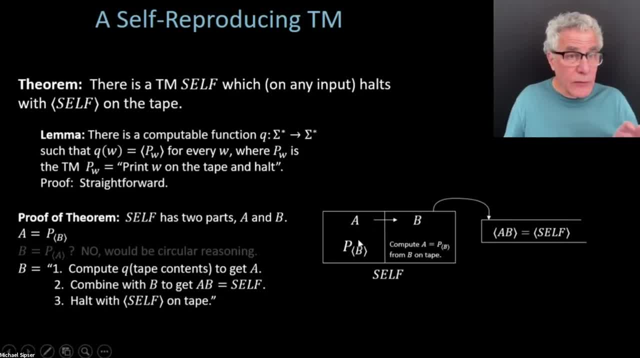 So first you produce B, Then you can figure out, then you can obtain A. There's nothing circular in this argument. I don't know if that's helpful to you, but you may need to mull it over Or maybe it'll be helpful from the next slide. 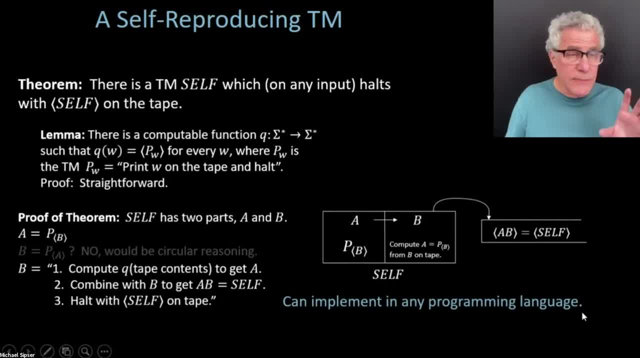 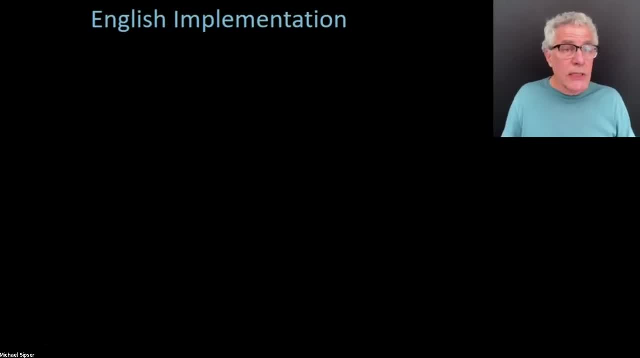 So let's go there now, OK. So, as I'm saying, you can implement this in any language. In particular, you can implement it in English, OK. So let's just shift gears. Let's talk about writing down English instructions. 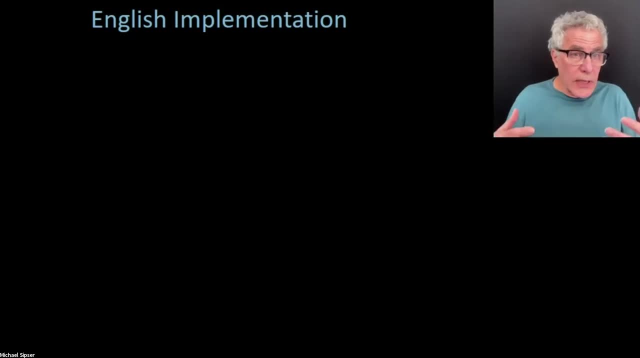 And then I'll show what happens if you carry out those instructions. So let's see. Start simple. How about the sentence write hello world. So an obedient person reading those instructions would then write hello world on their paper or wherever. OK, 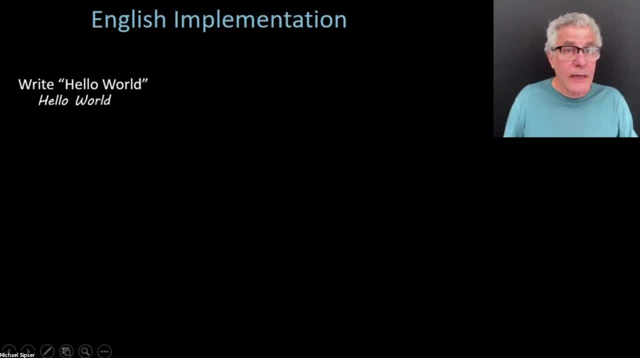 Fine, Hopefully you get the idea. So now, what I'd like Here is another sentence, another instruction: Write this sentence, And the reader- the obedient reader- would then, OK, write this sentence. This is the kind of thing I'm looking for. 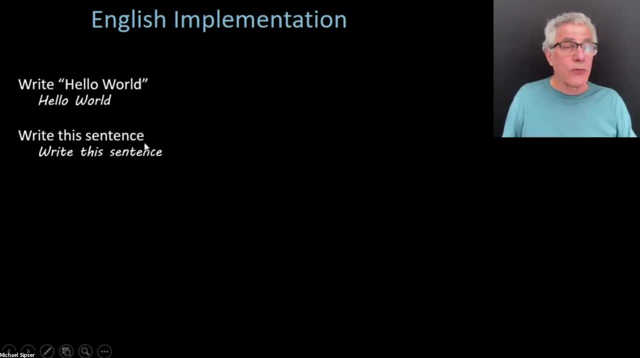 Here is a sentence which instructs the reader- The reader- to make an exact copy, But I don't like this one, Even though it does in a sense what I'm looking for, Because it kind of cheats When it has this. this refers to the entire sentence itself. 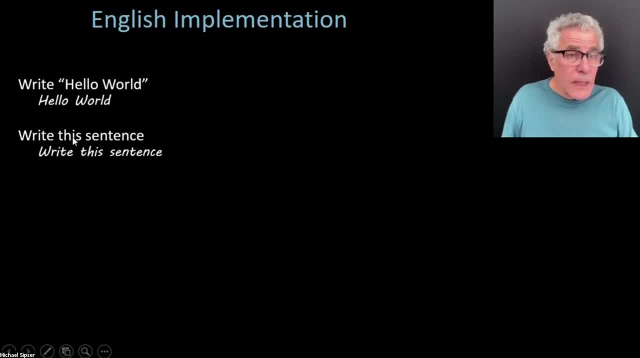 It's using, kind of implicitly here, a construct which a Turing machine does not have. A Turing machine does not have a way of accessing its own code. And in fact, really what the point of this whole theorem that we're going to present is that you don't need to have this self-reference as a primitive. 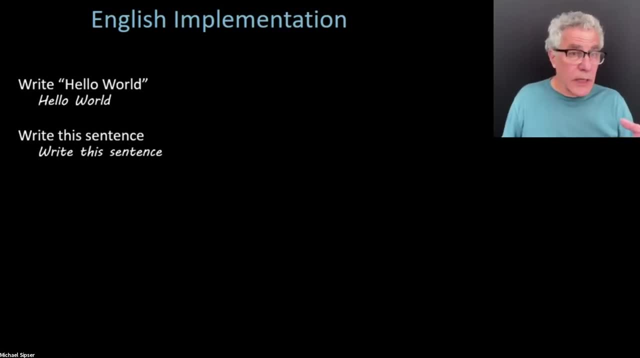 You can get that effectively using the procedure that I'm describing, which will give you the same effect. So you don't need it as a primitive. You can design some software, basically, which will give you the same effect. So let me show you how to do that in English. 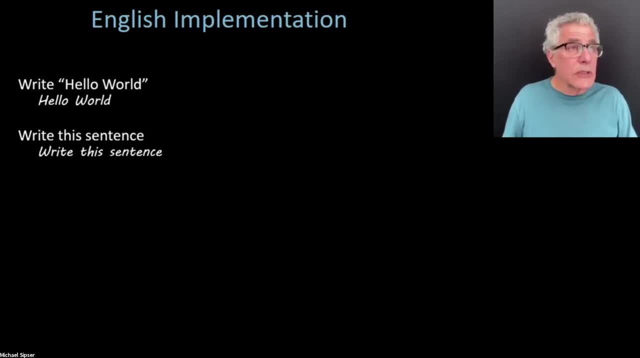 So let's look at a slightly more cheating. So Turing machines don't have the self-reference primitive, So let's look at another sentence here. Write the following twice the second time in quotes, And then hello world. So what do we get if we follow those instructions? 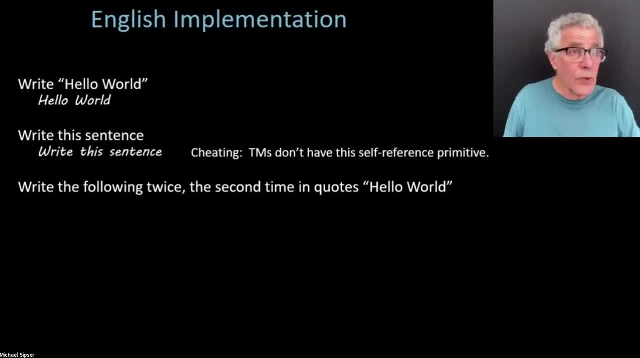 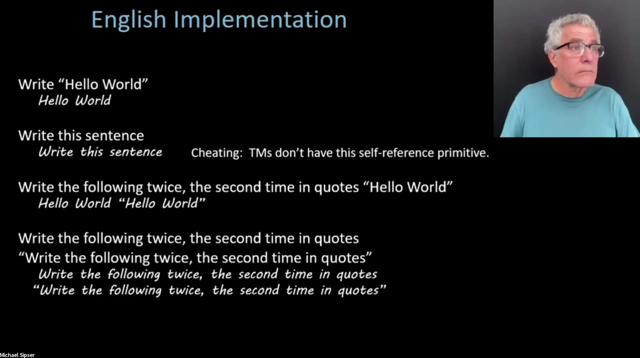 That instruction. Well, you get hello world and then hello world again, now in quotes. Hopefully not too bad. But now I'm one step away from doing the implementation of the self-reproducing algorithm in English. Write the following twice, the second time in quotes: 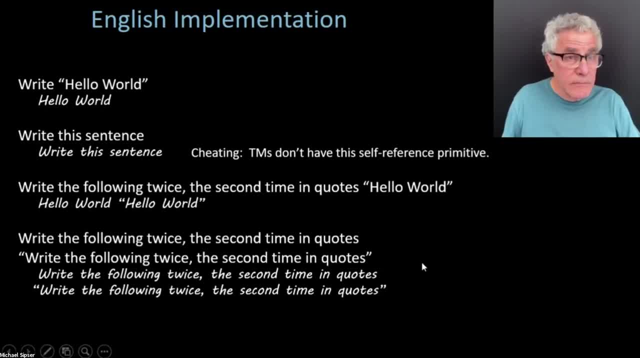 And then in quotes, And then in quotes the same text. Now, following those instructions, you get well, write the following twice: the second time in quotes, So that comes out here, And the second time you put it in quotes. 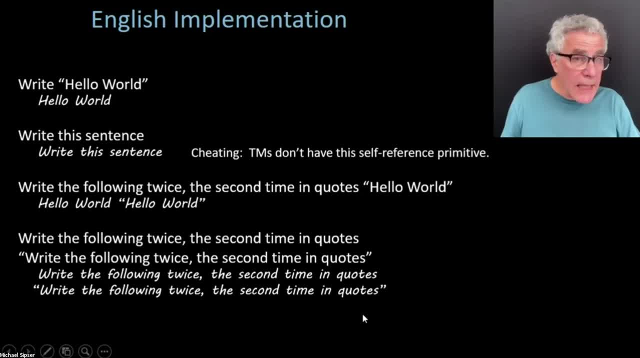 Just like you did with the hello world. But that's exactly what. here the output is exactly what the input was And there's, you know, even though there is a part of the sentence here which refers to a different part. So here the first part is referring to the second part. 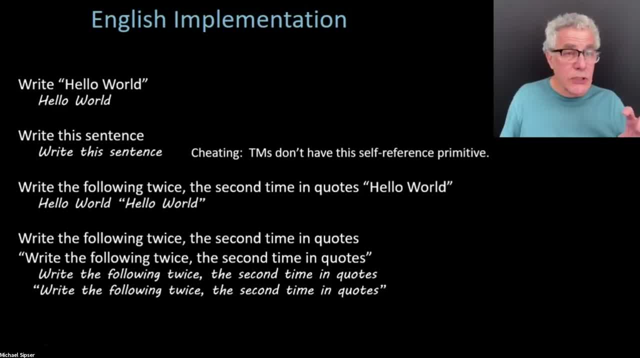 Never do I have to have the sentence referring to its entirety. You know there's no part of the sentence here that's pointing at the entire sentence, And so this here manages to get the effect that I'm looking for, where the output is equal to the code but avoids having the self-reference. 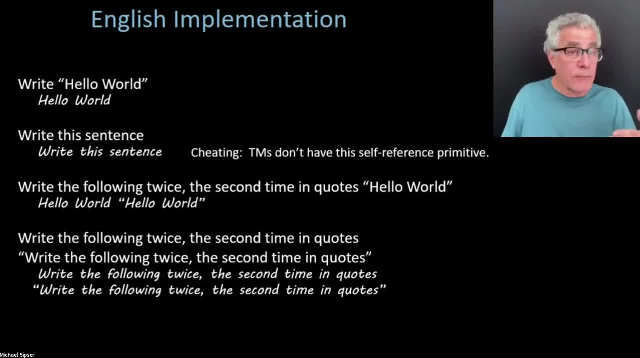 There's one thing that's referring to something else but not referring back to itself. OK, So let me just see here. So here is sort of- I'm going to have a check-in on this in a minute, So I'm going to try to contrast what's happening here. 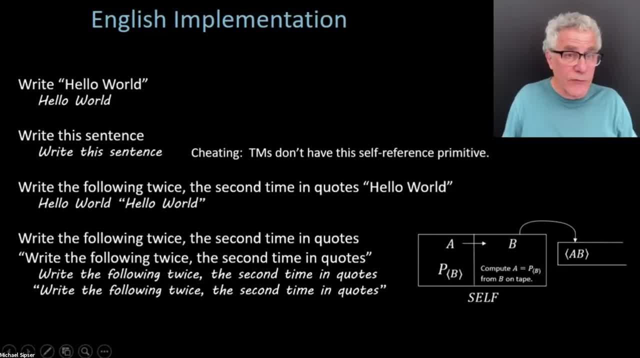 with what's happening in that turning point, And I'm going to use the machine self that I had from the previous slide. OK, So why don't you mull this over? And I'm going to give you a check-in to see. 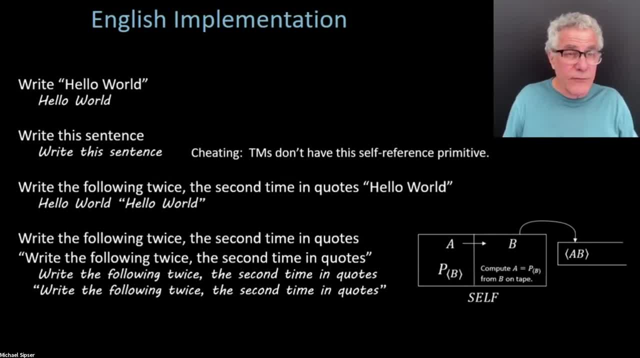 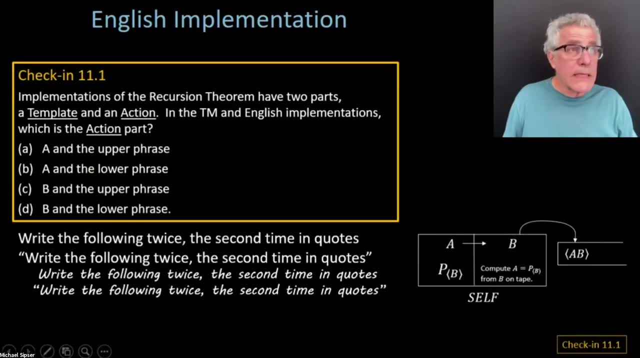 This is a little bit of a challenging check-in, But let's see if you can figure your way through it. OK, And basically it says so. really, what we're doing here is called the recursion theorem, as you'll see. 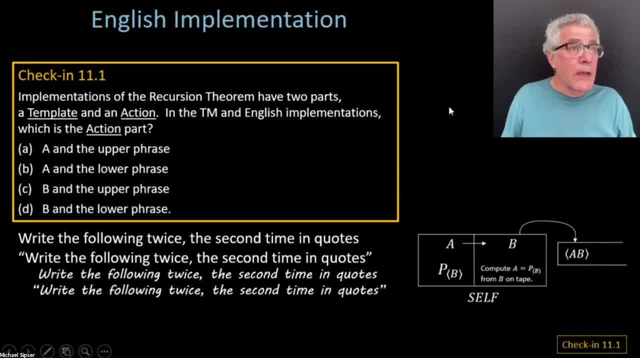 We'll actually present the recursion theorem formally on the next slide. But here, In both of these cases, we kind of have a template part and an action part. In both cases we have, there are- two parts to the instructions: the template and the action. 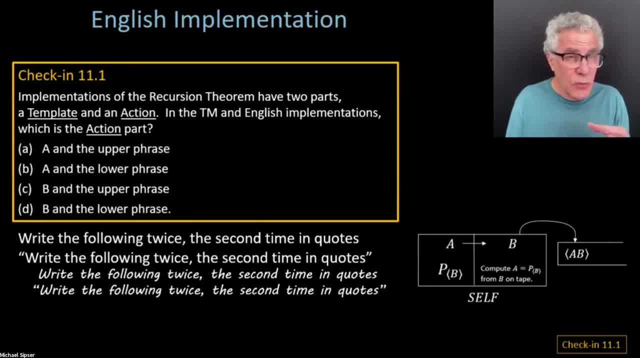 OK, So I'm going to leave it to you to try to imagine which of those which is which in each of these two examples, And then I'm going to ask you to pick in the Turing machine which is the action and which is the template. 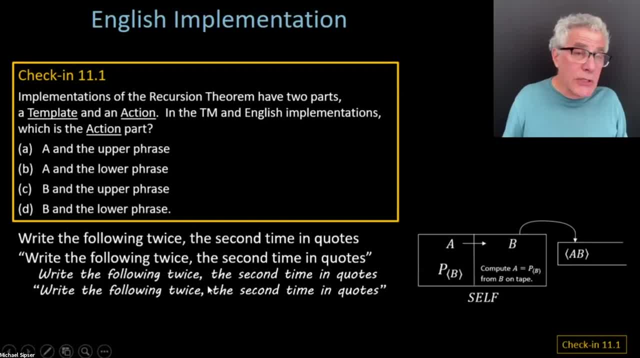 And in the sentence, which is the action and which is the template. The action is the part that where there's some interesting sort of stuff, instructional stuff, happening that you have to carry out. The template is really basically just text or just a string. 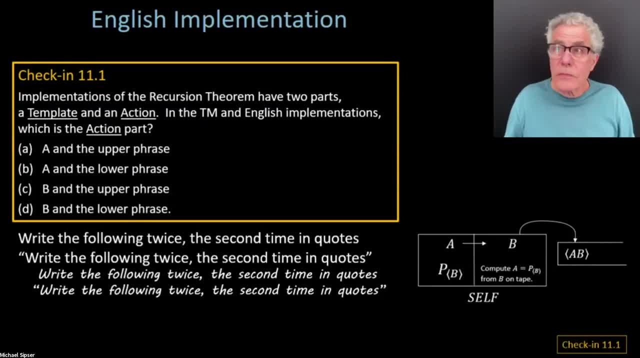 OK, So let me pull up that poll See what you think, Because I'm asking you now to indicate where is the action part in both of those cases? What is the upper phrase and lower phrase, I mean, of the sentence here? 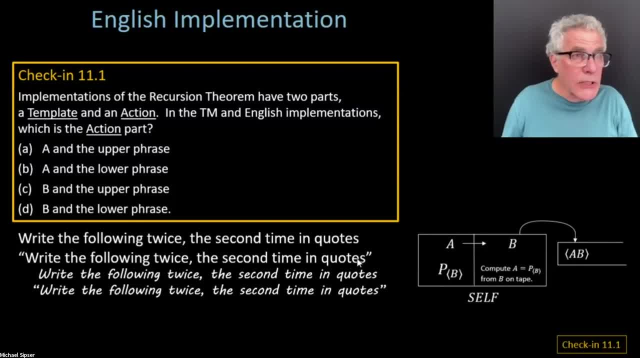 So write the following twice: This is the upper phrase And the part in quotations is the lower phrase. Sorry, OK, Almost done here. Five seconds. Few of you have not answered it yet. Answer it One second to go, OK. 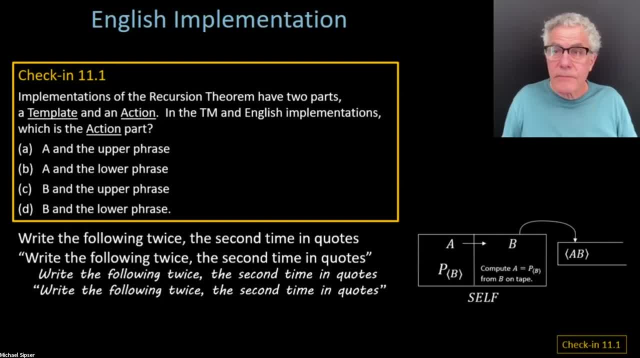 Here we go, Ending polling. So the majority here is correct. I would say in the English sentence: here the action part is the first part, That's where you actually have being directed to do something. The second half of the sentence, the lower part of the sentence. 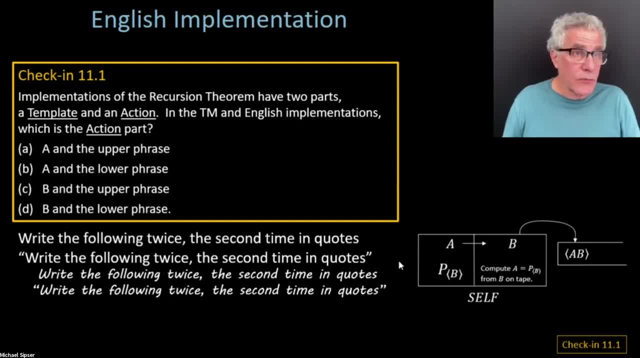 is just a template written. This is just some string. here There's no action really being directed. It happens to be the same as the top, But this could have been just hello world. This could have been anything, And then the upper part acts on that. 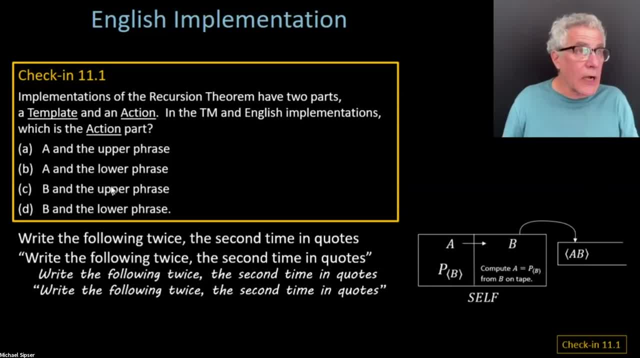 So the upper part is the action part, So it's the upper phrase. That's the relevant part. Now in the Turing machine it's kind of the. in a sense it's the other way around. The first part is really just the template. 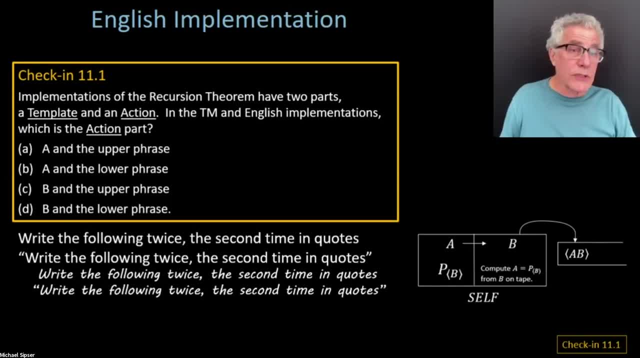 The second part, B, is where you're doing some actually work on the template. You're taking that basically text which could be anything- A could be anything- And you're You're looking at that template and reconstructing what A was. 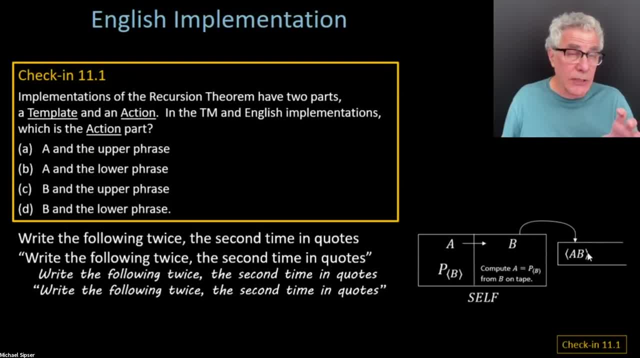 from that string that appears on the tape. So B is actually the one that's doing the work. So it's B and the upper phrase It's part C, is correct, Okay, So let us continue then. Oh, I want to mention here: 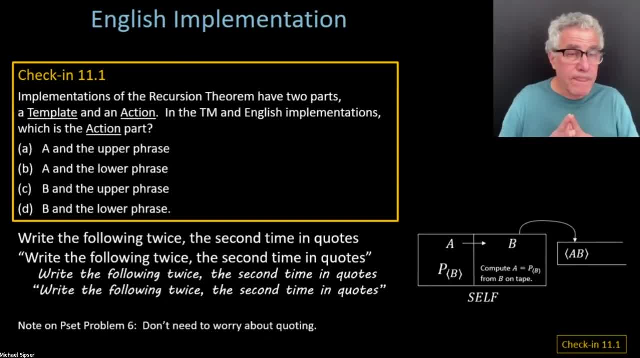 Problem six on the P set. So you know your job really is to implement this in. you know, if you have a programming language and you love that, you like, you can, you can. it could be Python or whatever your favorite Java, whatever you like. 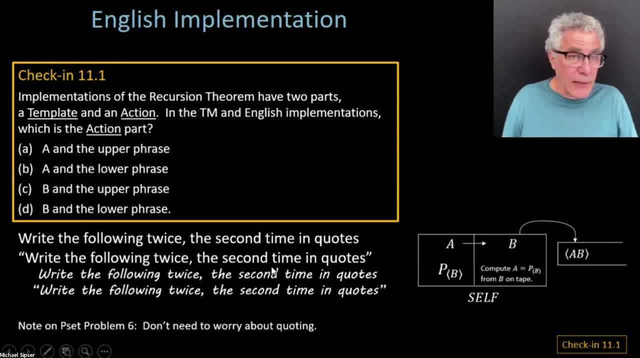 you can implement this. If you don't know any programming languages, then just make up some sort of pseudo programming language and implement it there. Let me point out that Getting the quoting Right Is a bit of a pain, Because you have to kind of escape the quotes and so on. 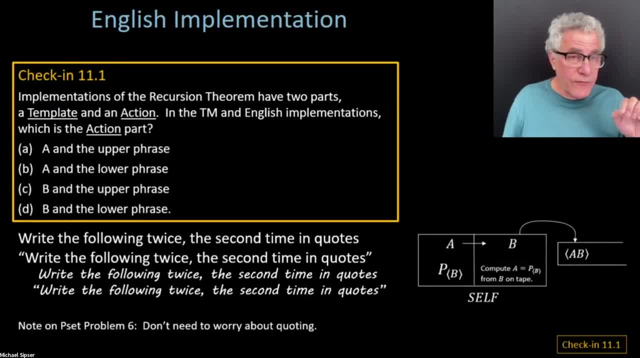 I'm not going to be fussy about that. So you can still get full credit even if you don't get the quoting part quite correct. do your best. I think it's an interesting problem to try to solve And if you, 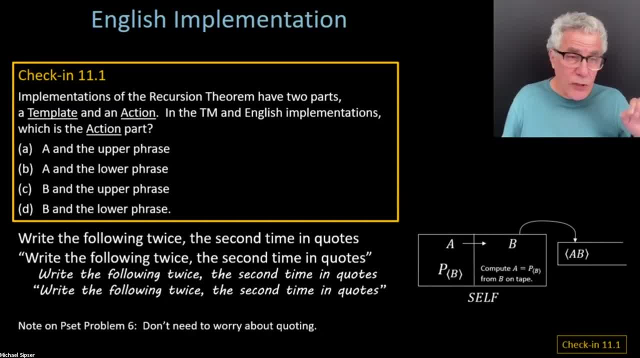 you know if you struggle with it for a while- you know you know it's slippery- It's the kind of thing you have to. you know. you know you can easily spend a couple of hours on this problem because it's. 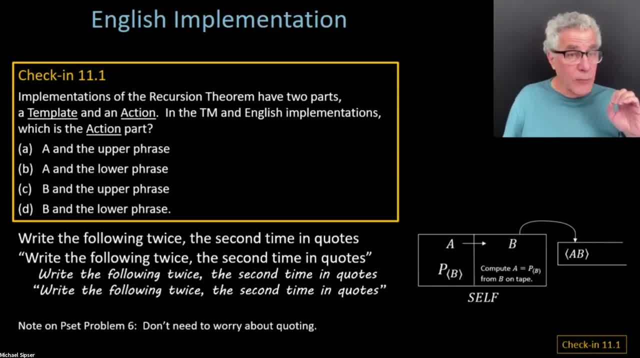 it's, it's. it's a bit tricky to manage to make a program which prints itself out, which is what the task of problem six is. on the on the piece set, But don't fuss about too much on the quoting. 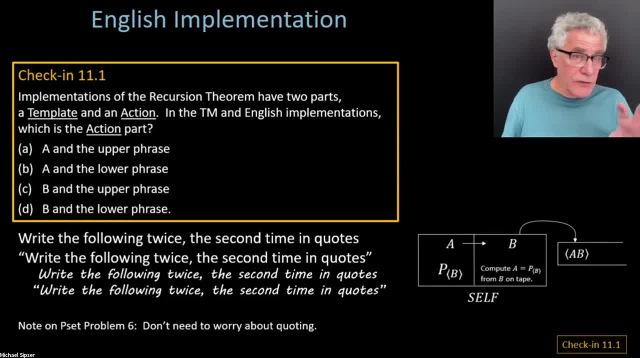 If that's the only thing that's hanging you up, try to get the main structure of it, which is fairly simple actually, And if you can't get the quoting part to work, you know I'll ask the graders not to penalize you for that part. 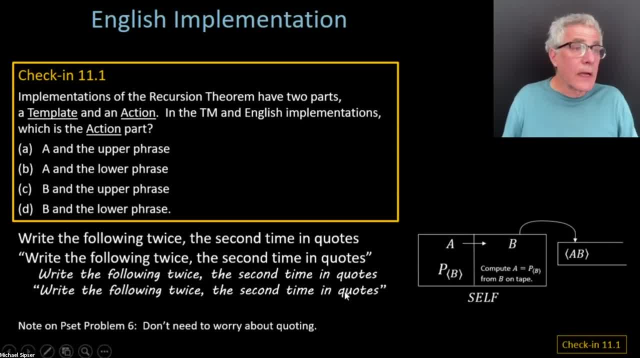 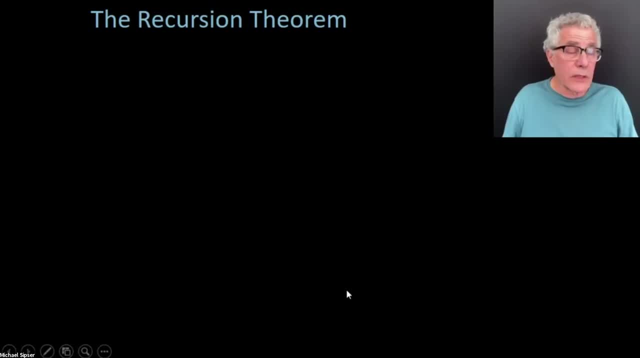 Okay, Let's. let's then look at this sort of the more formal version of what we've just done and really kind of also taking it to the next level, Because being able to print out a copy of yourself is is kind of a curiosity in a way. 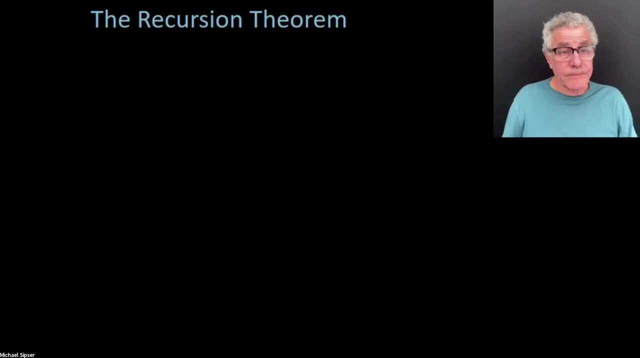 But you know, the recursion theorem says: not only can you make a machine which prints out a copy of itself, but you're going to actually make a copy of yourself. And so you know you're going to have to make a copy of yourself. 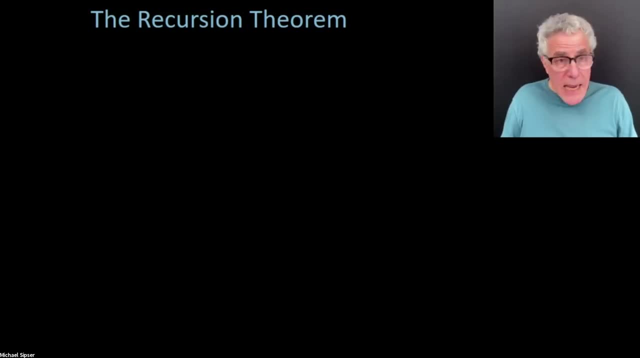 And so you're going to actually make a machine which can obtain a copy of itself and then do some computation on that copy of itself, on its own description, which actually turns out to be a useful thing to do Once you have access to your own description. 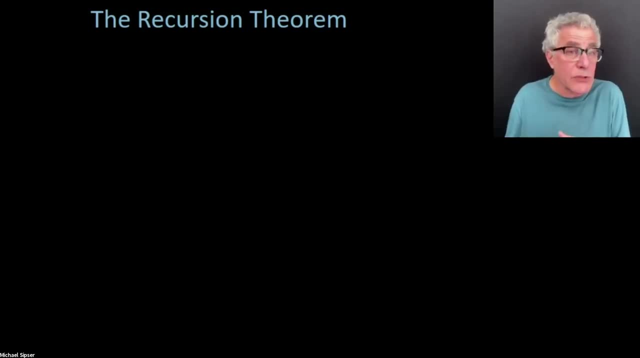 as we'll see from some examples, then you can do some, perhaps some interesting things with that. Okay, So basically, what, what, what? the recursion theorem is a kind of a compiler. It allows you to have a new primitive when you're writing Turing machines. 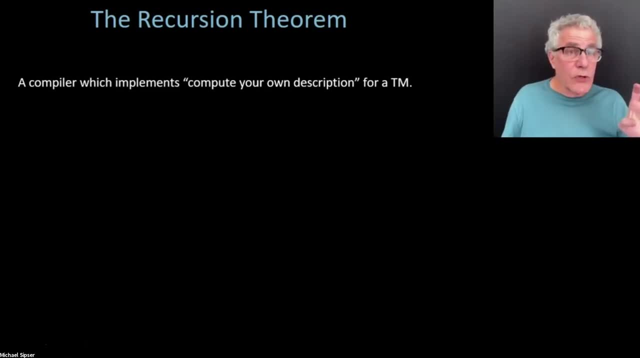 Which is compute your own description, And the recursion theorem will implement that for you. Okay, So the technical form of the recursion theorem is going to look a little bit counterintuitive. perhaps. Let me put it out there: If you, if you struggle with a little bit with the slide, 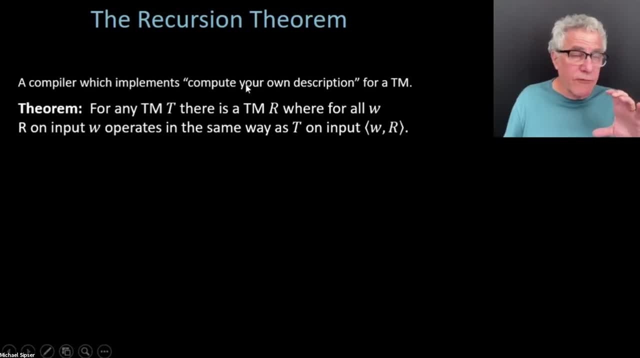 don't sweat it. The main thing to remember- and we'll see from examples- is that you can compute your own description In a Turing machine And that's going to be allowed as code. Okay, So what? the way we're going to do this is. 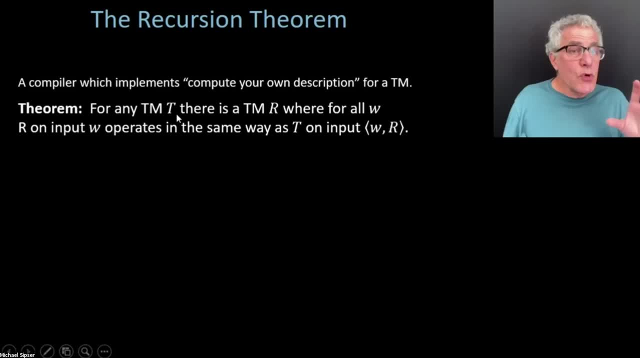 what the recursion theorem does for you is. it says you can write a piece of code here. Let's call it a piece of Turing machine code algorithm- algorithmic code called T, And T is going to get transformed into a new machine. 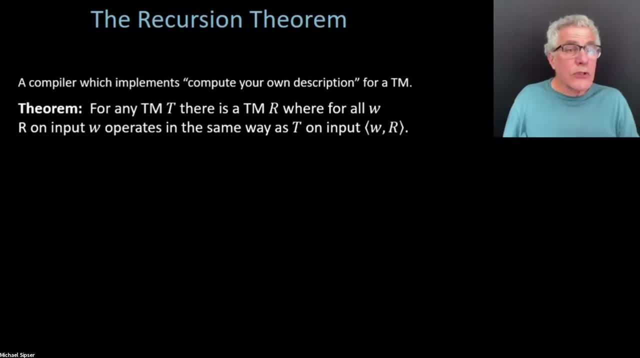 R, And R is going to get provided a copy of the program itself, which is just a description of R, for free, But otherwise it's going to act exactly like T. So R is going to act exactly like T, except R is going to have provided a copy of R. 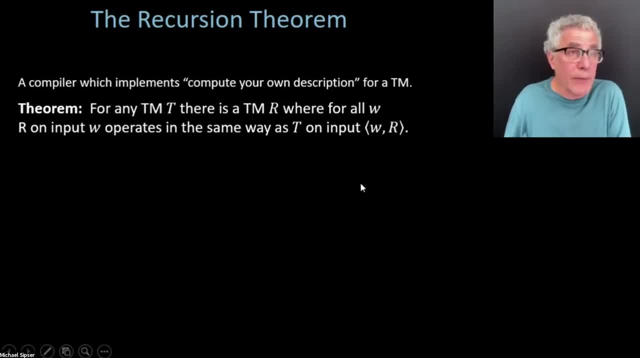 And that's what the theorem shows you how to implement. So let me, let me just see. So, for any machine T, there is a machine R, which, for any W, which is going to be the input to the input for R, 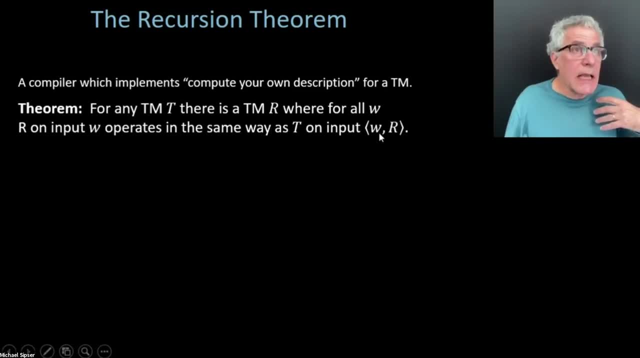 R on W operates the same as T on the input, with W where it's given, where it's given R. So R is going to be be getting access to R without it's going to be configuring obtaining R by, by calculating it. 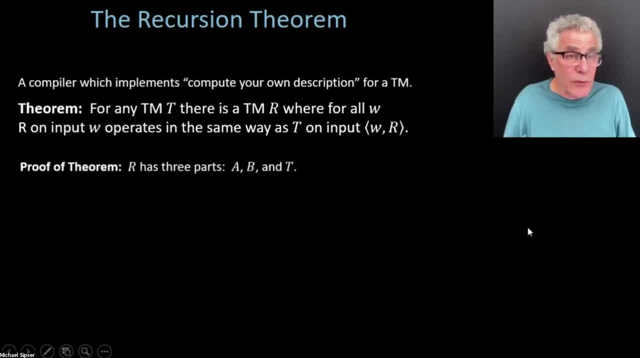 Maybe it'll be clear from the from the proof. I always struggled with how to explain this clearly, So now the proof of this is going to be very much like the proof from two slides back, except there's going to be three parts. 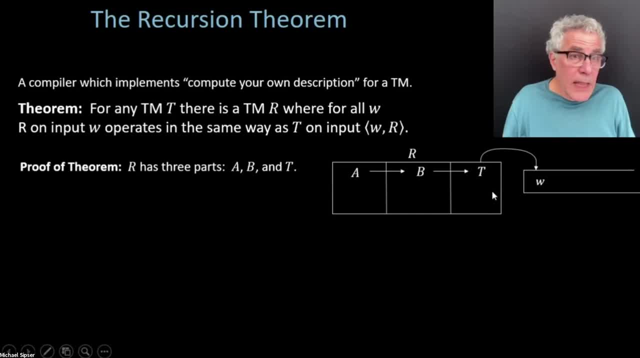 There's the, the part T that you're going to provide, And the T is going to be the Turing machine code that says: get your own description And you don't have to worry about how that happens. The compiler is going to add on the A and B parts. 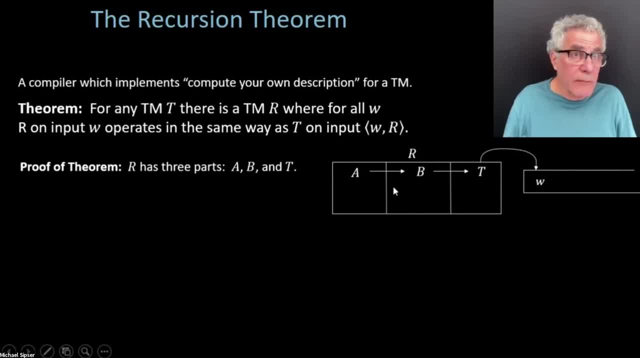 which is going to get the whole description of the whole thing, which is R, and feed it into T As if T- you know T had it as an input, So it's T is going to be allowed to get its own description now and operate on. 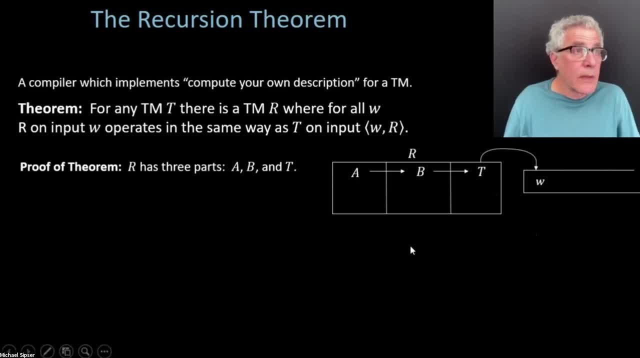 now operate, does its thing, you know, on the input W. So the way it's going to work, so T is given, A is going to be, as before, the description of B, now with T. So when A, when A is done. 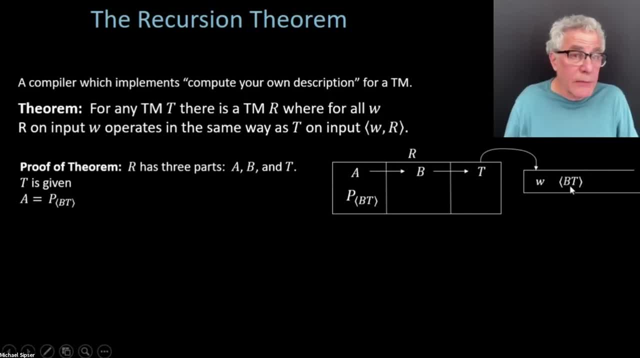 it's going to produce BT sitting on the tape next to the W. B is going to now figure out what A was from the BT sitting on the tape. Okay, And then it's going to combine that to get ABT, which is R. 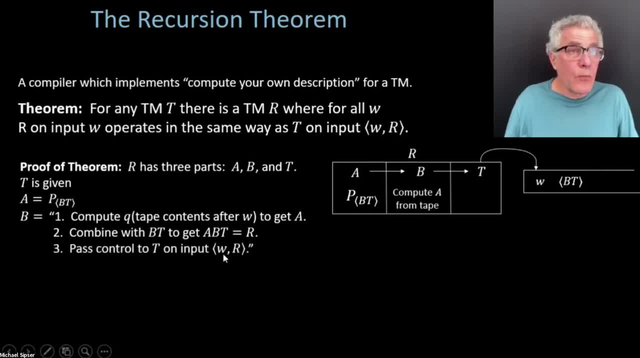 And after that it passes control to T with, with W and now R sitting on the tape. And now T. T is going to have its own description, but don't forget, now T has been modified to be R, So it's not that T is going to get T on the tape. 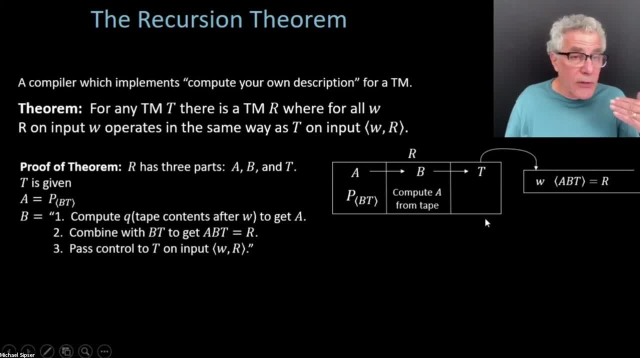 It's going to for this to make sense, this is this is going to be now the new machine: R and R is getting is appears on the tape And now the code that you provided T is going to get is going to now going to get to operate on that. 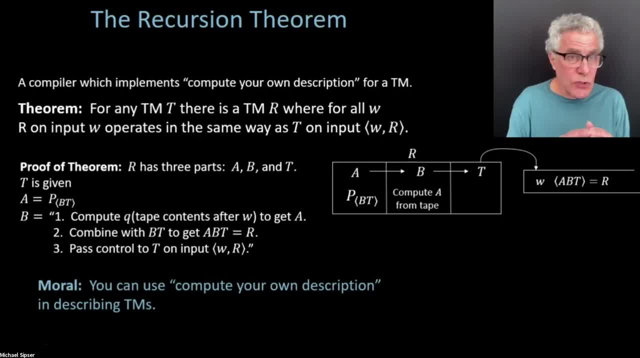 Okay, If you didn't get that, I'm not. so I'm not worried. The main thing is that you can use compute your own description When you're describing Turing machines. That's what this thing is telling you. I think it'll be. 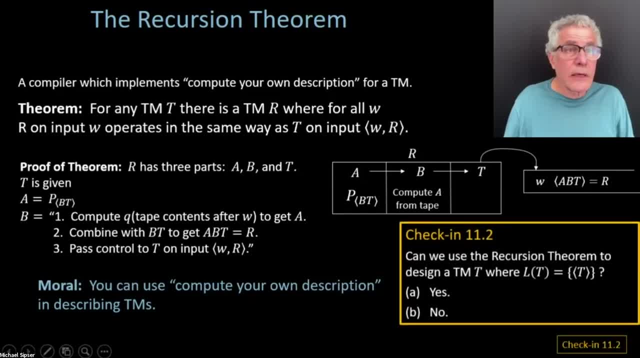 Oh, there's a check in here, Yeah, So I don't know, Let's, let's do this one kind of quickly here. Can we use the recursion theorem to design a, a machine T, which, instead of producing its own description? 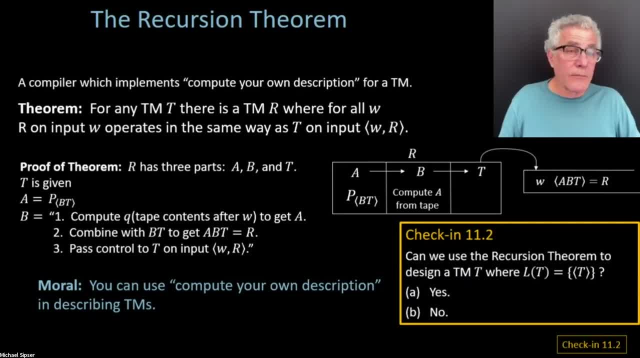 recognizes, recognizes, recognizes, accepts only only its own description as an input. So the the language of this machine is going to be simply the one string, the description of T. So can we make it a machine, T, which does this? 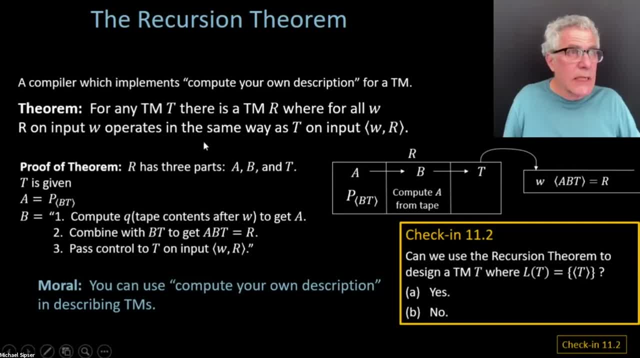 No, I now I'm looking at this. check in This T here is confusing with that T. It's not the same T, It's bad. I should call it M, Design a machine M, where L of M is the description of M. 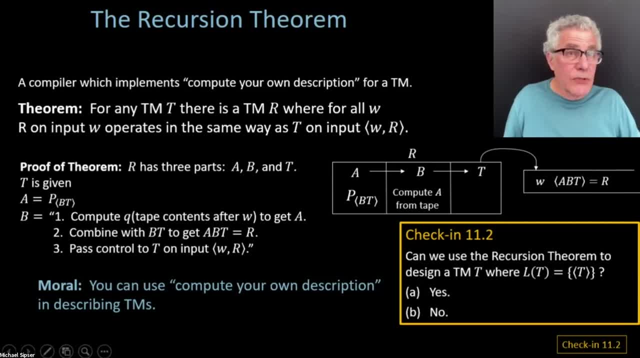 And can we use the recursion theorem to do that? You know what? what I would ask you to do is think about it in this context. You can use compute your own description when you're writing the code for this machine. If you could do that. 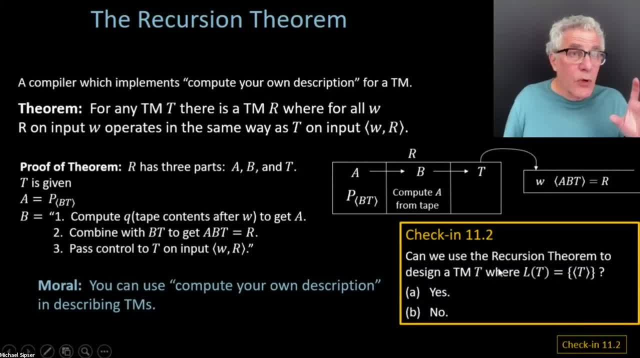 could you make a machine which just accepts strings, which happened to be their own description? This is supposed to be easy, but I think it ended up being a little bit more complicated than I wanted, So so I think that's what I wanted. 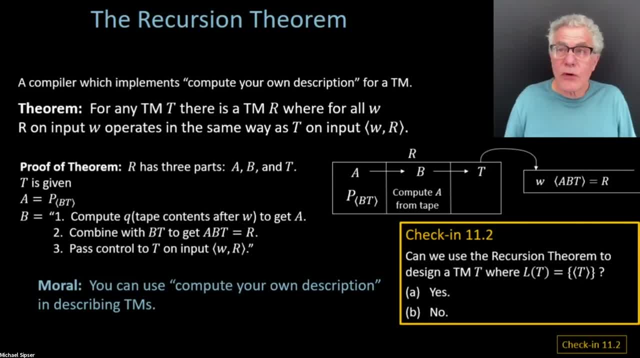 Okay, Launch polling. Make your best guess. I think you all can kind of see what I was kind of leading you, leading you, leading you along the path here, Yes, So I think you're pretty much all are getting it. 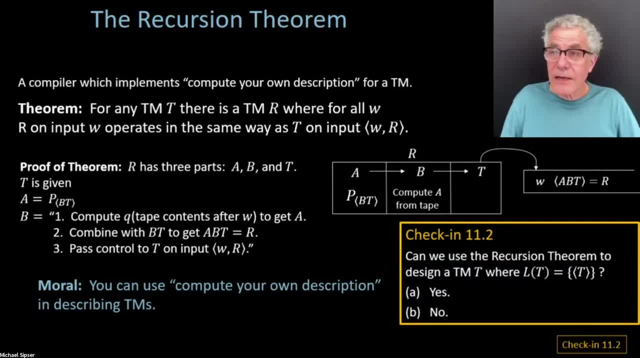 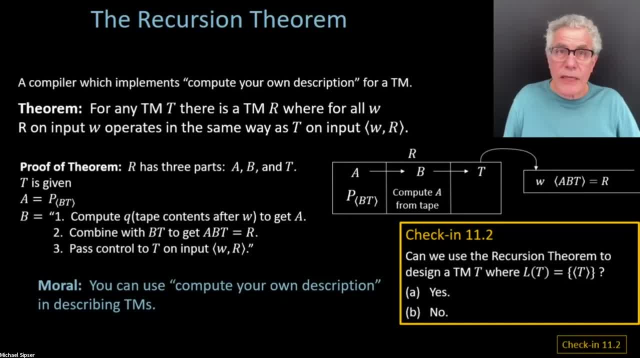 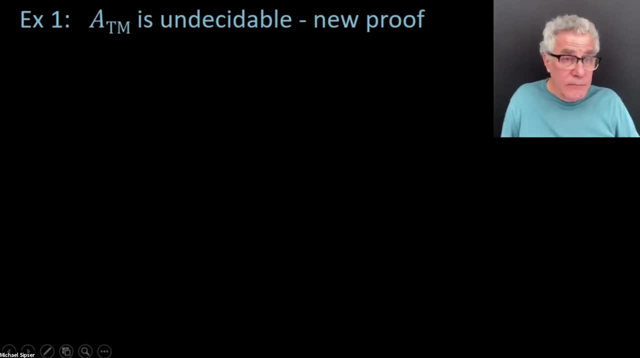 I'm going to end it. So the correct answer is yes, as I was hinting at. So let's. I think maybe this example would have been better after the next example, and then we're going to have a break. So here is a new proof that ATM is undecidable. 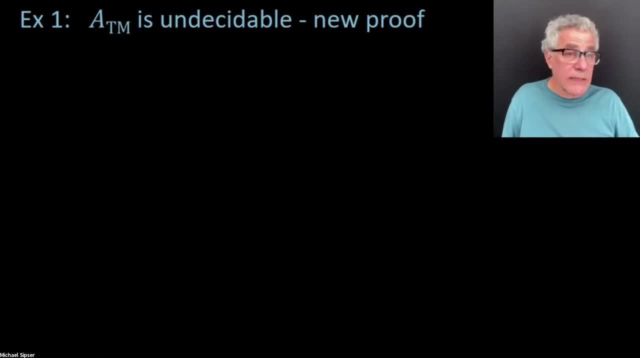 but now using the recursion theorem, And this is going to give you a nice example of how we use the recursion theorem in action. Okay, So remember, we spent, you know, half a lecture or more with a proof by diagonalization as our first example of an undecidable problem: ATM. 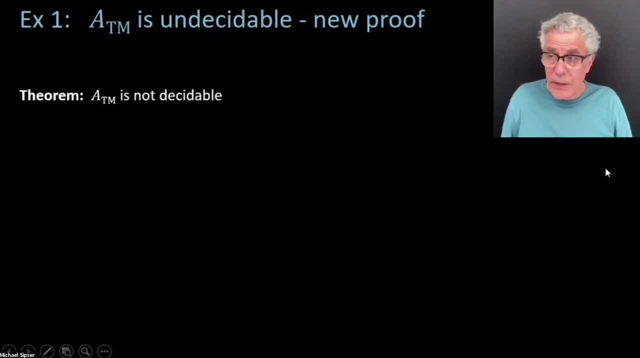 We subsequently showed other things undecidable by re, by reduction, But for the very first example, we use that diagonalization. Now I'm going to give you a new proof. Okay, So proof by contradiction. assume we have a Turing machine that decides H, that decides ATM. 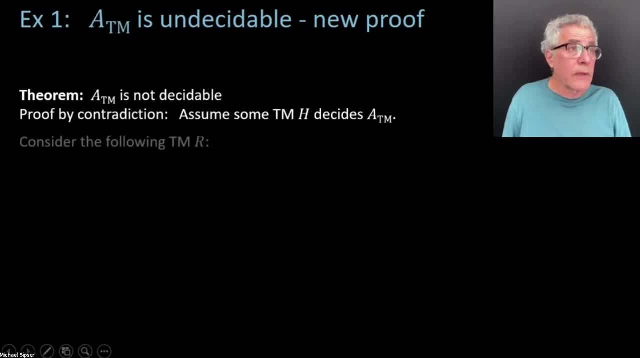 It starts the same way that diagonalization proof went, but now I'm going to make a new, a machine called R, So this is going to be different. This is different from the earlier proof. R says on input W. I get my own description. 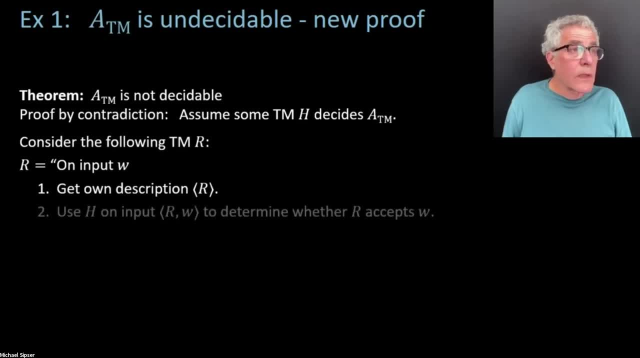 use the recursion theorem. That's the way these things always start. Now I'm going to use H. Now that I know my, my own description, I'm going to feed. I can ask H. I can feed. R, W, W was the input here. 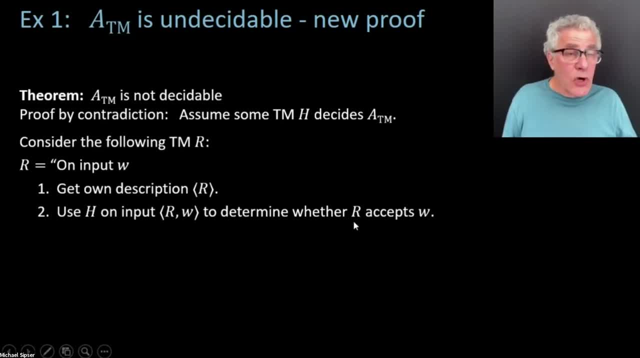 I can feed R, W into H to determine whether R accepts W. That's what H does. H will tell solving ATM. H will tell this: tell this machine whether R accepts W. R is the machine we're writing. However, that is the machine that. 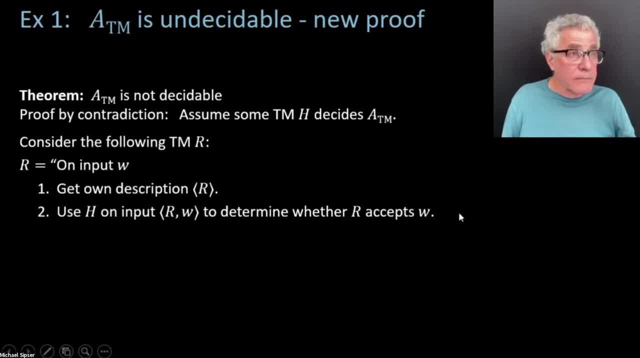 that is the machine where we're currently. that's currently running. So H R now uses H and it knows what it's supposed to do. H is going to say: well, you're going to accept W or you're not going to accept W. 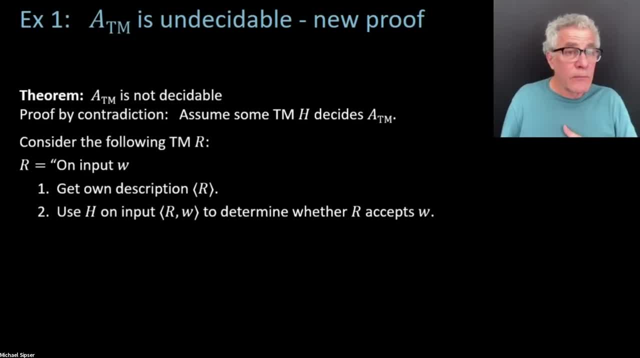 That's what H is assumed to be able to do. But then what? what is R going to do after that? R is going to do the opposite of what H says It's going to do. So if R H says R accepts W. 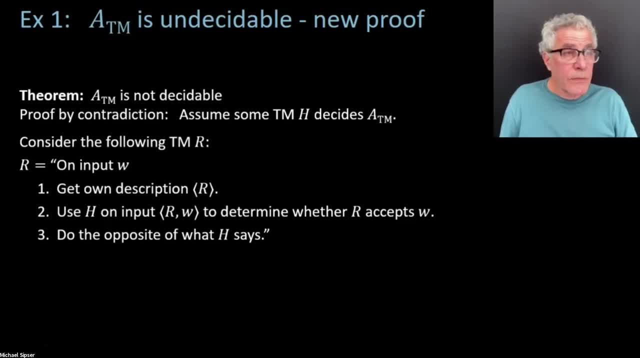 then R is going to reject W. If H says R doesn't accept W, you know, rejects it by looping or halting, doesn't matter, H just says it rejects, Then R, it's just, you know, it's just going to accept. 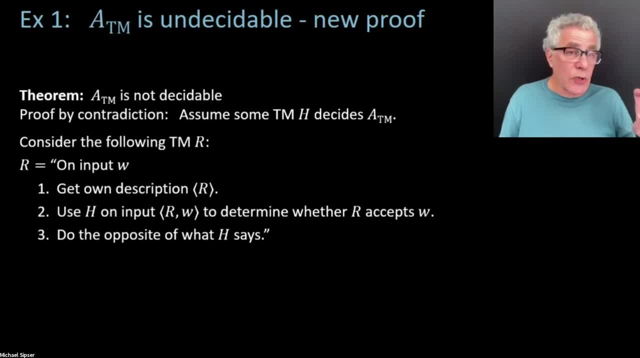 So whatever H says, R is going to show that H is wrong. So that's a contradiction. It says that H cannot be deciding ATM. So you know, if you step back and think about what this is here, that's that whole diagonalization proof. 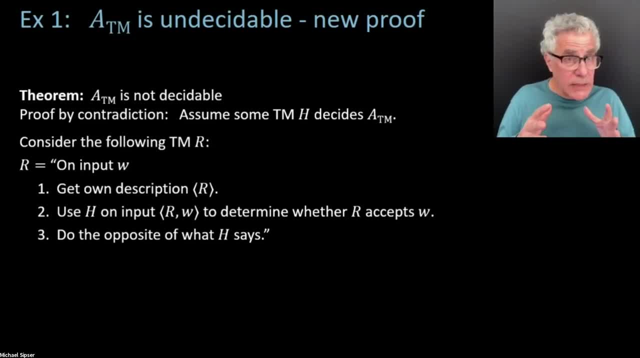 you know, in, in in one line. basically, we've done that proof in a different way, though There is some similarity here. I don't want to say this: We've totally reinvented things and done it totally differently, but it's kind of. 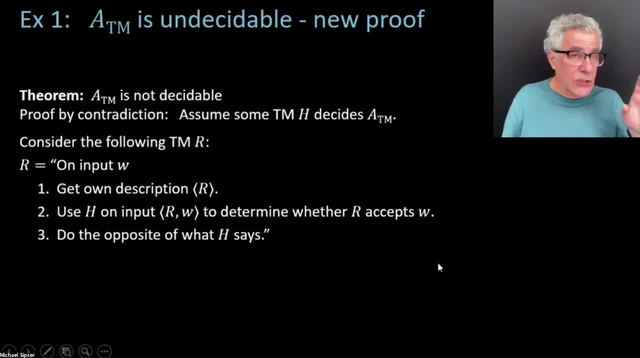 in some ways sort of gets at the essence of the diagonalization In a certain sense. But anyway it gives you kind of a new, very short proof that ATM is undecidable. So I think that's kind of a cool thing. 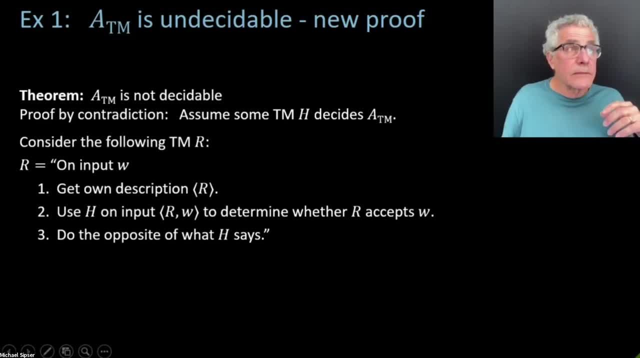 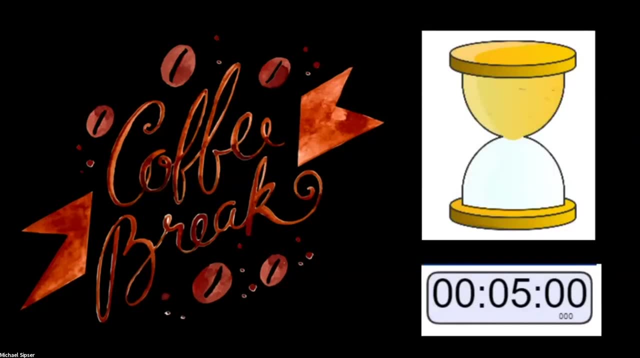 So why don't we take our little coffee break here and you can feel free to ask questions during the break? I will start my timer going and we'll be back continuing lecture in five minutes. Okay, So questions. So we're getting some questions. on when I said, 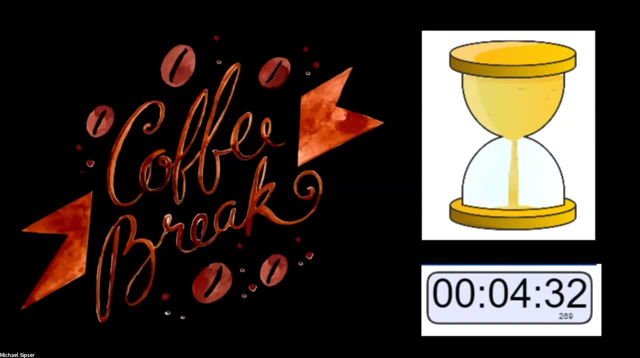 we don't have to worry about the quotes. when we're making the solving problem six on the P set, Somebody says: can we just say print ABC instead of print quotes, quote ABC and it'll print ABC. Yes, you can, Don't worry about the quotes. 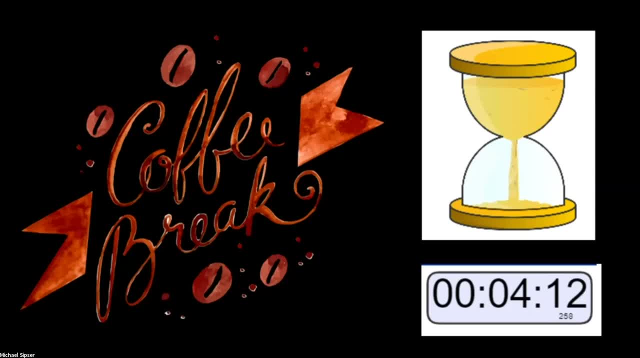 If you know, I think it's kind of you'll. you'll see a challenge if you want to try to make get the quotes to work, but it's also kind of a pain. So yeah, you can just kind of ignore the quotes and I'll ask the graders to. 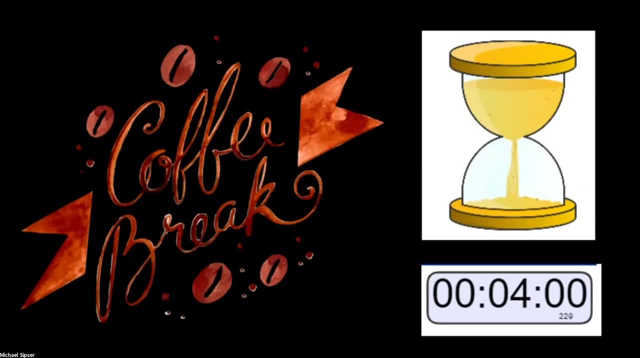 to mark that, to mark give that for marks there. So don't that that's any reasonable interpretation. We'll, as long as you get the rest of the concept right, We'll be fine. Let's see Somebody is asking in the recursion theorem. 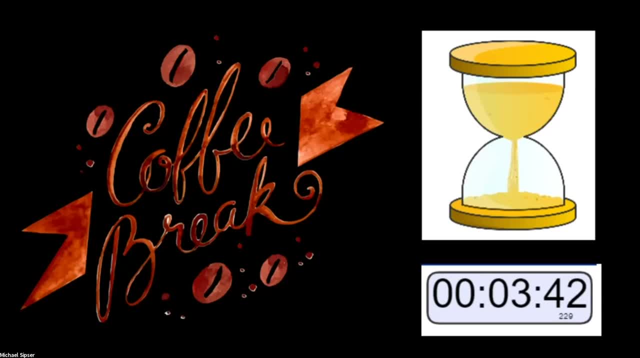 why doesn't T get the description of T instead of the description of R? because we're producing the. the machine that's running is R back back in the previous slide, two slides ago. So if I, if R got T, it would not be getting its own description. 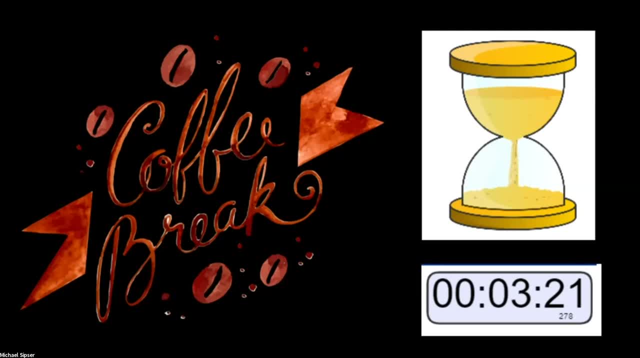 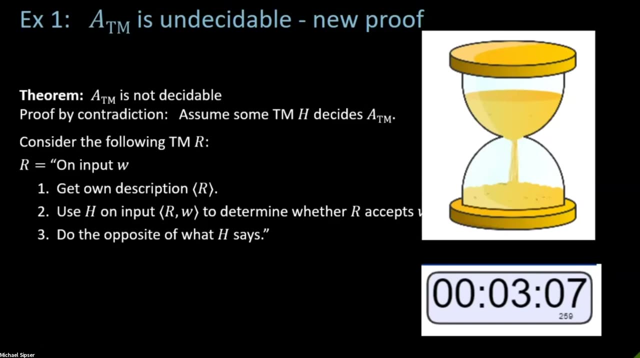 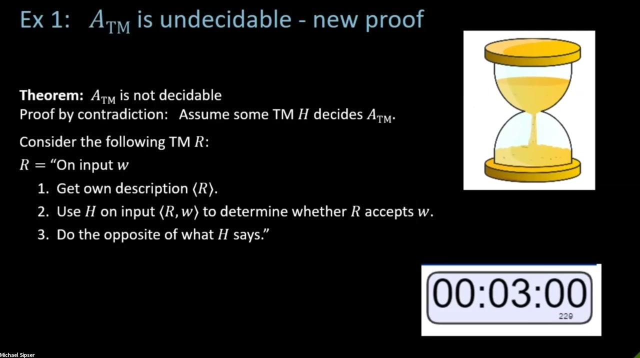 be getting the description of some other machine. So you need to think about what what we actually need to have happen here in the proof of the recursion theorem. but it needs to have R, not T. Let's just see, if I can. why does R do the opposite of what H says? 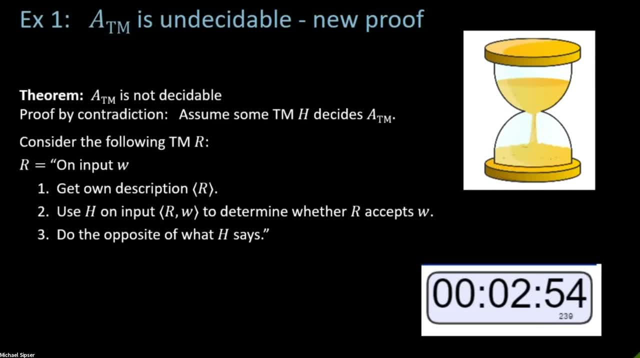 Why does R do the opposite of what it says? Well, first of all, I'm so. here's the code: arc. You know we're assuming we have H, I'm going to design R to do anything. I want to satisfy the proof. 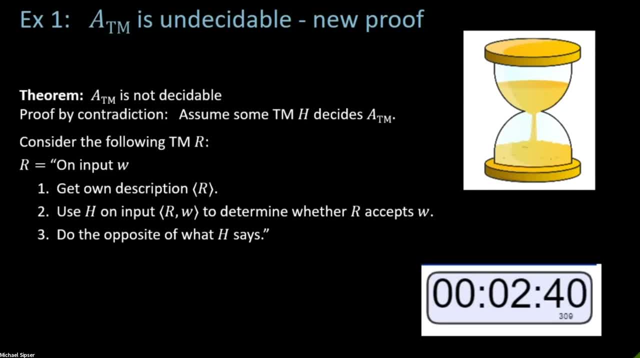 And R here is designed to do the, the the opposite of H. So I'm asking R, I'm programming R, to find out what it's what H predicts it will do, and then do the opposite. You know, you know. 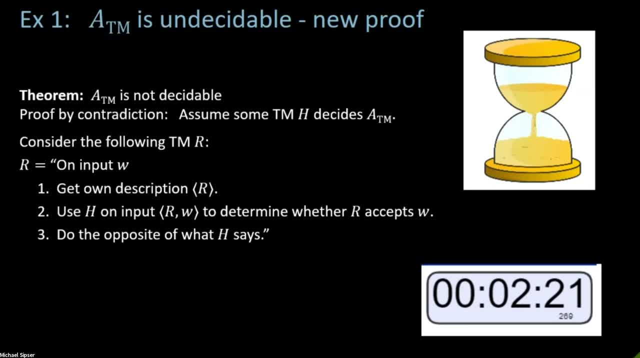 I, I'm going to do something like this. Suppose somebody says: you know, I have a crystal ball which is going to be like the role of H, He said, oh really, That's. that's kind of cool. I don't believe you. 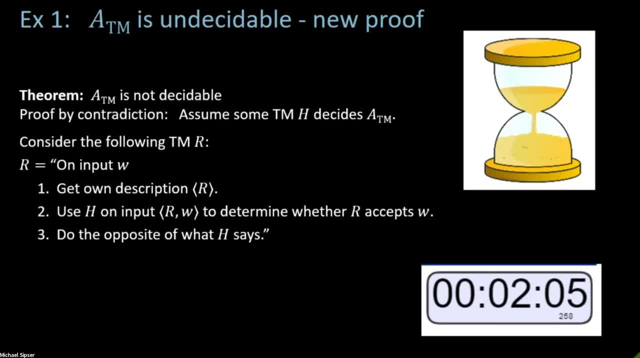 but it still sounds interesting. And the person says: yeah, I can see the future. I, you know, I know what you're going to do in five minutes And in fact I see that in five minutes you're gonna say hello and you can say: well, you know. 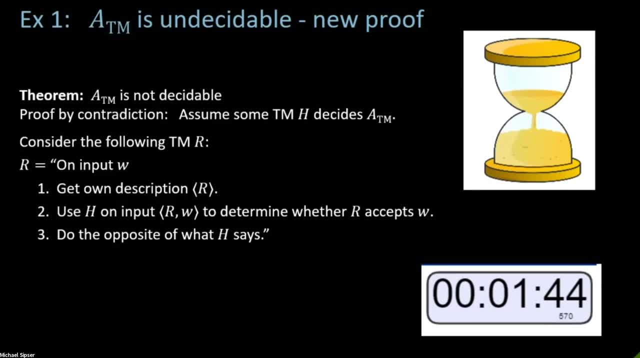 well I'm. you can think to yourself: well, this person is nuts, I'm not gonna do that, I'm just not gonna say hello. and then you know the, the genie there with the, with the crystal ball, you know, waits five minutes and you don't say hello and 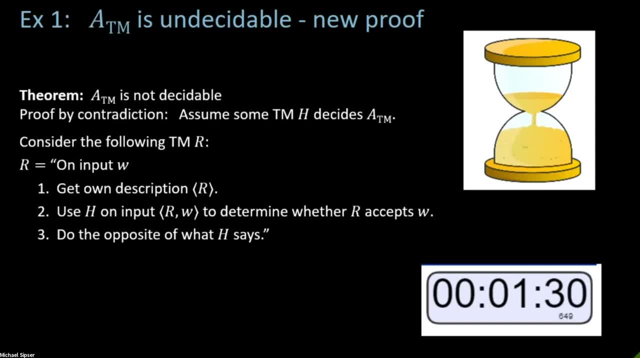 then you've proven that the crystal ball doesn't work. it's very similar, okay. okay. I'm not gonna explain how we can do the combining itself. that's just it's. you know it. I just want to explain at a high level. that's just going to be messy. 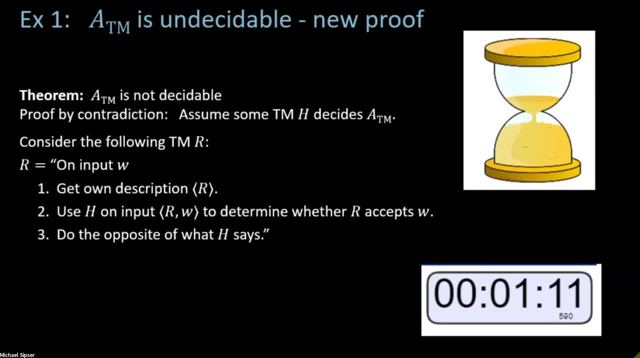 so because I said we somehow going to combine in self. let me leave that as a conceptual level. um, okay, how does this idea work for Turing machines? I don't really understand that question. how does this work? idea work for Turing machines are decidable. you'll have to think about it and you'll have to think about it. 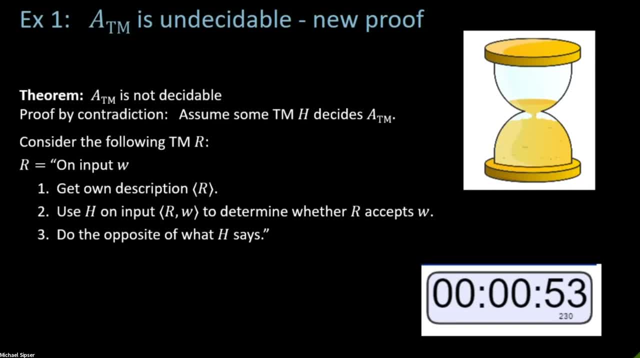 and you'll have to resend that because I don't understand the question. can I explain? use your own description. so what, when I, when you write code that says get your own description, after that code executes, the Turing machine has appears on the tape, like magic, the description of its own code you know, say sitting: 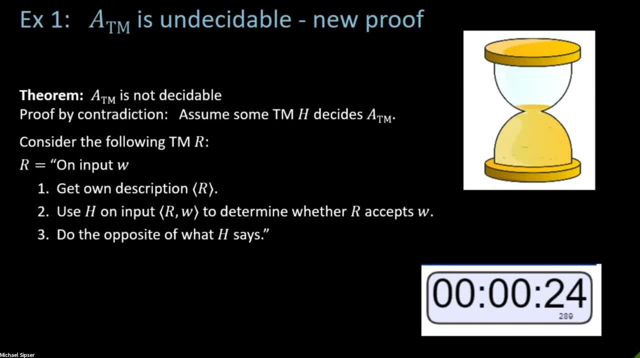 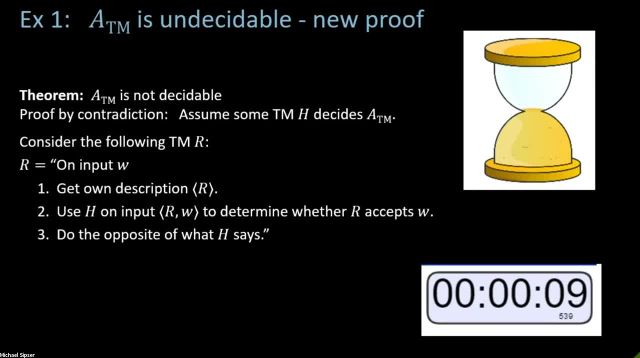 I still don't understand the question. so for problem six, is it enough to attach code? if your, yeah, you can attach code for problem set six, problem six and that's. that's good enough, and or, if you can explain, it's also good, like usual, do we worry about? 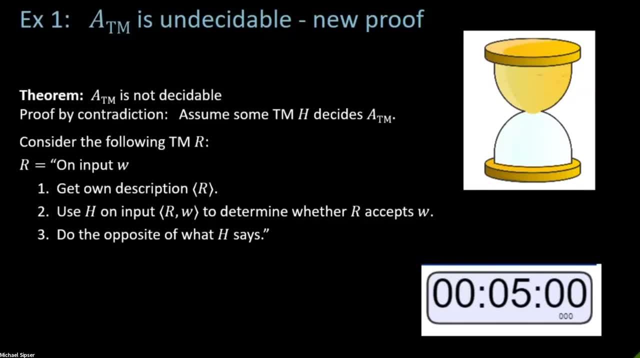 tabs and new lines. no, okay, we're gonna have to defer the rest of the questions. don't forget, we have zillion questions here which I didn't get to. okay, last last one here: why does programming R to do the opposite of age? is that a contradiction? well, H is predicting that our accepts, but our doesn't accept, so H? 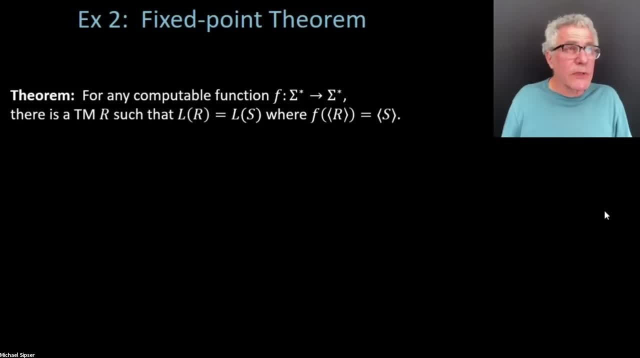 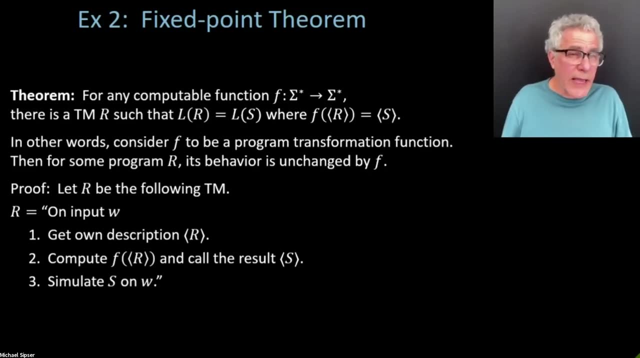 is wrong. we're a little short on time, let me skip this one. you can look at this on your own. I mean, this is proving sort of the cool fact that if you have a- I'll just say it- a high level, if you have a, a program transformation, so if I 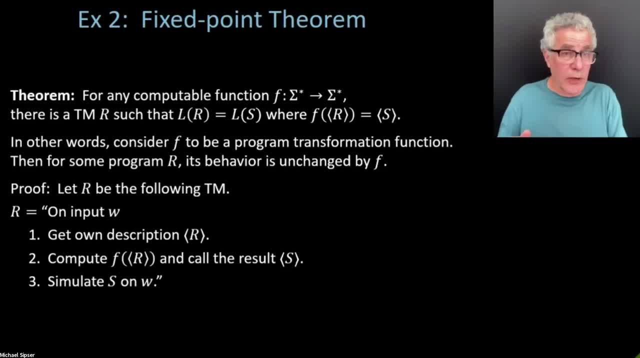 have some manifestation. there's no Chi here. it's all right if I have some transformation. so if I have some merchandise, that I have all these functions and I add these functions and these functions- method of transforming one program to another program. but it's done by algorithm, so an algorithmic way that 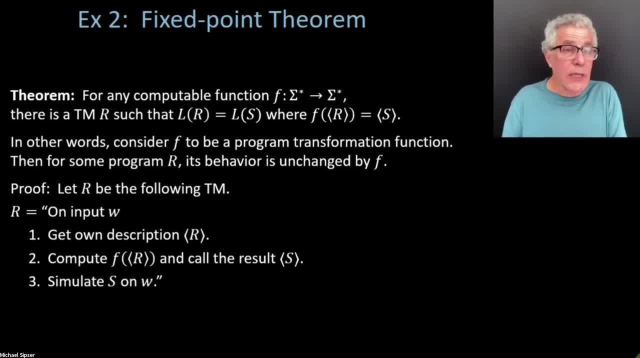 transforms one program to another program, There's always going to be some program whose behavior is unchanged by the transformation. That's called the fixed point theorem. So there's some program whose behavior doesn't change, No matter how you try to transform programs. 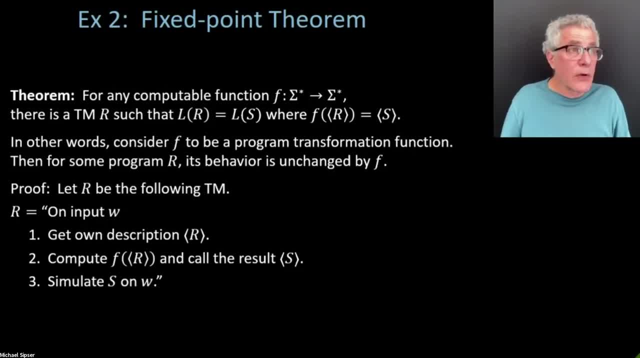 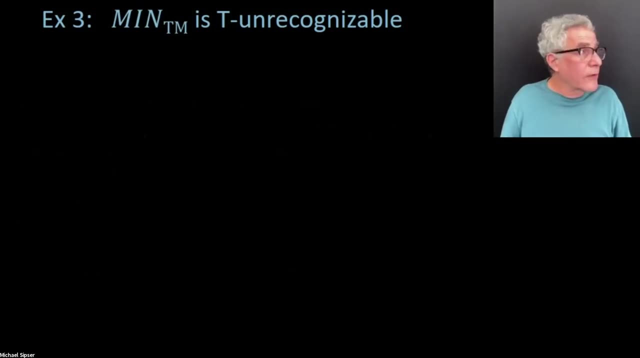 easy proof using the recursion theorem. You can look at the slide offline separately if you'd like to see how that goes. It's pretty simple. Here's another exercise of the recursion theorem. So if I have a, let's say, a min, 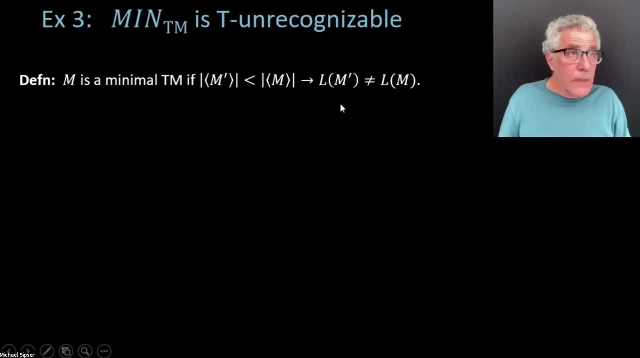 the concept that a Turing machine is okay. Now, a Turing machine is minimal if its description is the shortest among all Turing machines which behave the way it does which are equivalent to it. When I was an undergraduate, I took a programming class. Some of us sort of enjoyed writing short programs. 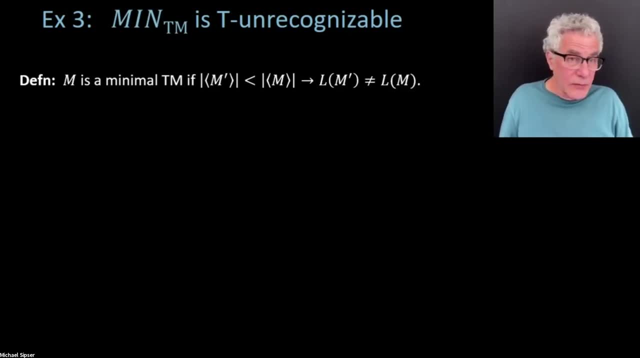 to carry out the exercises. Probably these days that's forbidden because it just encourages bad programming style, But anyway, and so you kind of won if you found the shortest solution for a given programming exercise. It was Heapsword, I remember was one of the ones. 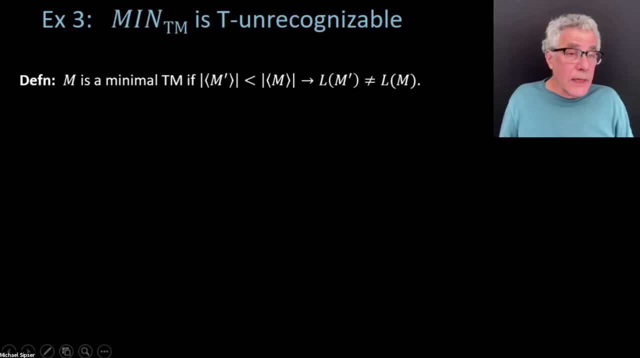 that we had to do. So. this is sort of similar. You might imagine that people try to find the shortest possible universal Turing machine. So shortest in our sense is in terms of whatever encoding method we have in mind. a machine is minimal if there is no shorter program which is equivalent. 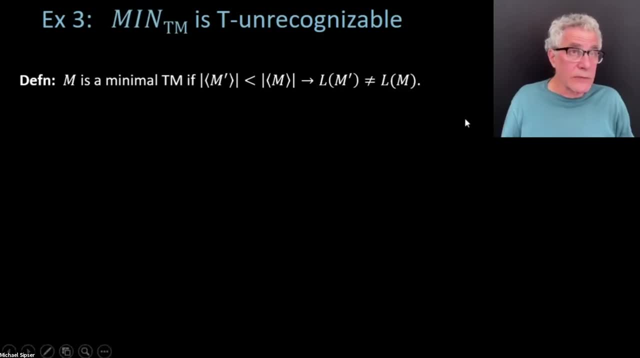 using our encoding system, whatever it is. So anything m is minimal. if anything that has a shorter description has a different language, OK. So let's look at the collection of all descriptions of minimal Turing machines And I'm going to prove that that language is unrecognizable. 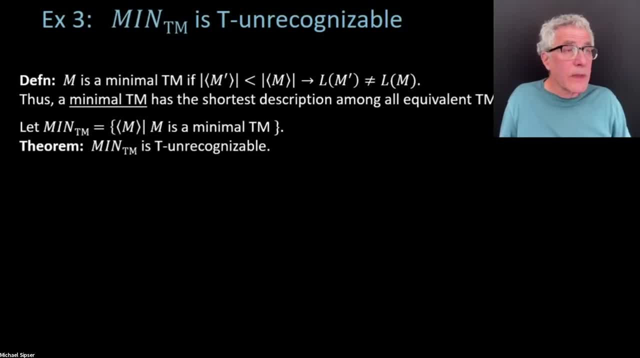 I'm going to do it using the recursion theorem. It's kind of a cool exercise And you can actually use it to prove something more powerful, But let's focus on this theorem for now. So Assume, Assume, Assume we have. 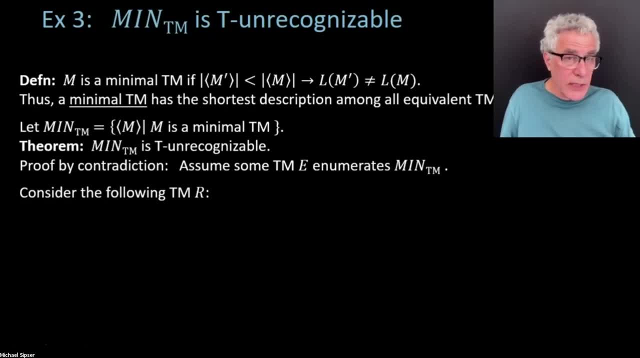 And it's also a little nice exercise about enumerators. I don't know how comfortable you ever got with enumerators, But I'm trying to prove this language here is not recognizable, And so remember enumerators. you can enumerate exactly all the recognizable languages. 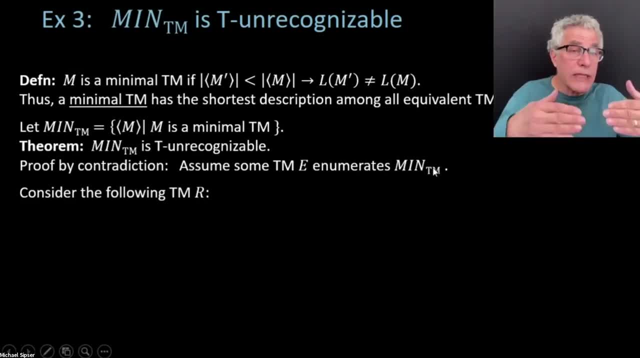 So I'm going to assume I have an enumerator for this language which just prints out all of the minimal Turing machines. So I have some enumerator. It's a program That prints out the descriptions of all of the minimal, the shortest possible, Turing machines. 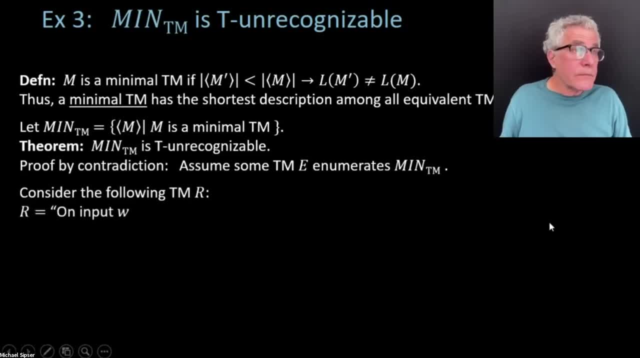 And now I'm going to get a contradiction. So we're going to take, build this Turing machine R, which gets its own description, And then it's going to start the enumerator until So it's looking at the strings this enumerator produces. 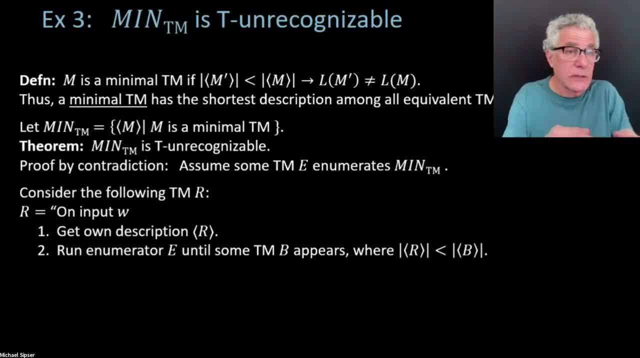 So this enumerator is producing these minimal Turing machines, one after the other, And then it goes back to the next. chunk, chunk, chunk, chunk, chunk. all these minimal Turing machines are coming out, And you keep looking at those until you. 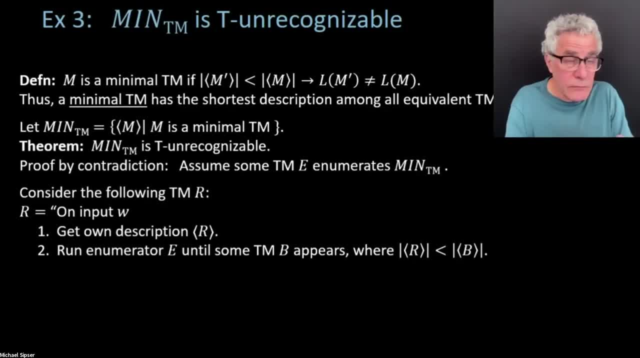 find one of them which is bigger than yourself. And how do you know how big you are yourself? From the description you're given by the recursion theorem. So you keep up printing out these Turing machines until you find one that's bigger than yourself. 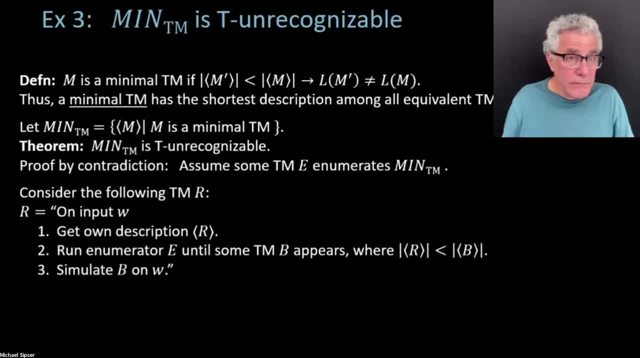 And then what do you do with that? You simulate that. So now, so what? Well, the point is is that you're going to be smaller than that machine that you're simulating, Because you waited to find a machine that the enumerator. 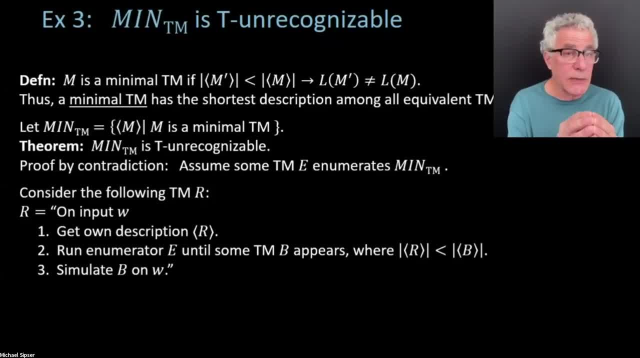 produced, which is bigger than you, So you're going to be simulating that machine that's bigger than you, And so you're going to be doing exactly what that machine does on every input, because you're always going to be simulating that same machine on every input. 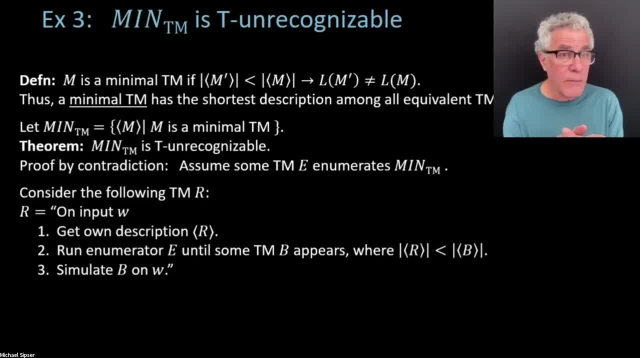 And so you're going to be equivalent. You're going to be equivalent to that bigger machine, But that bigger machine is supposed to be minimal because E is producing it, But here you are exhibiting a machine that's smaller than that, that's allegedly minimal machine. 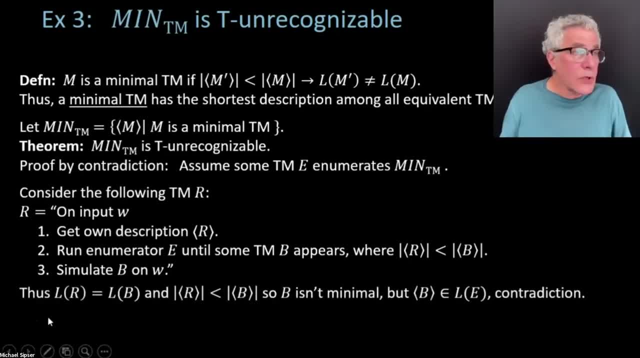 It couldn't be minimal. That's the contradiction. So the language of R- this machine I just produced- equals the language of B, because R ends up simulating B, But R is smaller than B because R waited until it found a bigger machine that's bigger than it. 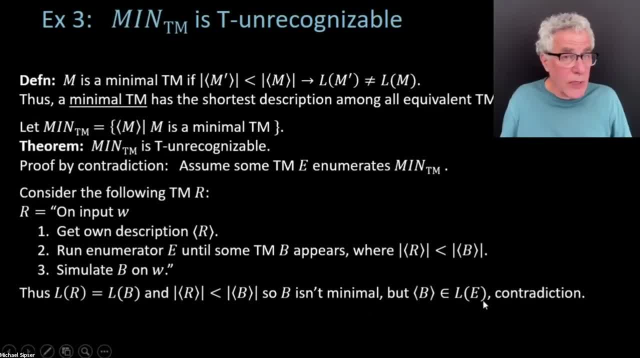 So B couldn't be minimal, But B was one of the machines that the enumerator produced. That's a contradiction, So let me do a check-in on this. I expect this is going to cause some of you heartburn, But let's do the best you can. 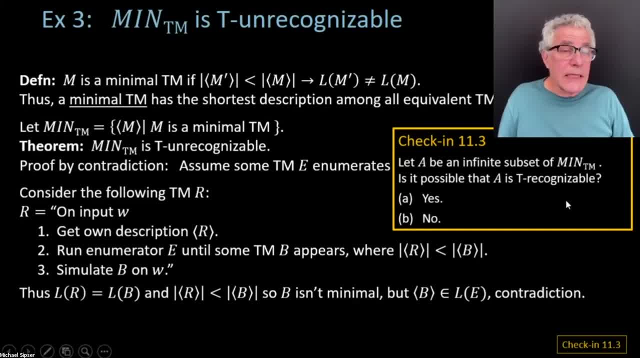 Suppose I have this collection of machines that I'm going to do to minimal Turing machines And I take some infinite subset of that. So now I'm not demanding that I have all of the minimal Turing machines, I just have infinitely many minimal Turing machines. 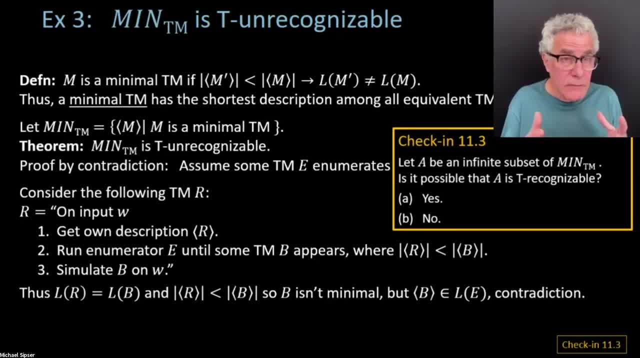 Is it possible that subset, whatever it is, could be Turing recognizable? Now, think about that. Now you can have languages which are not Turing recognizable that have infinite Turing recognizable subsets. Could that be for this language And maybe I'll give you a little it. 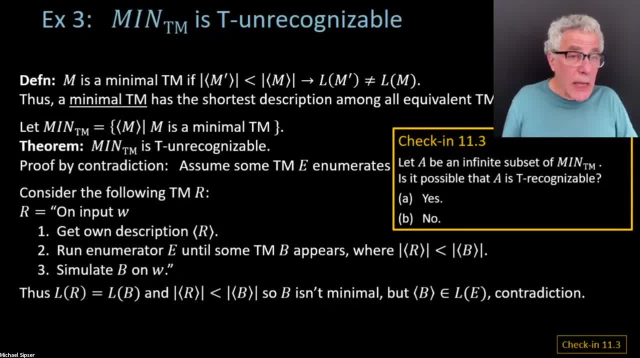 will be helpful to you to understand and perhaps apply, OK, The methodology that I gave you in this proof here And that might be helpful to you, But I can see this is not. this one is a bit of a struggle. OK, let's end it. 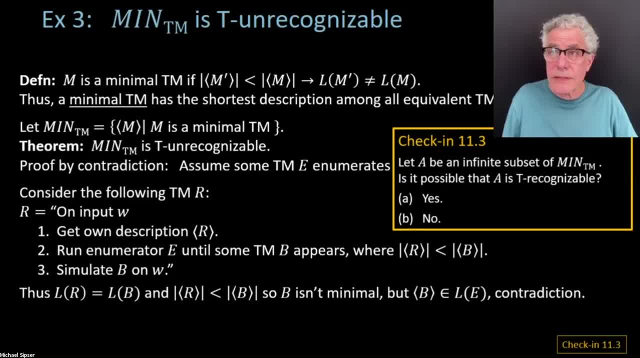 OK, two seconds, just pick something. All right, so the majority has the correct answer here. So, in fact, this proof would still work if the enumerator was enumerating an infinite subset of minimal Turing machines, Because all you need is to wait until one. that's. 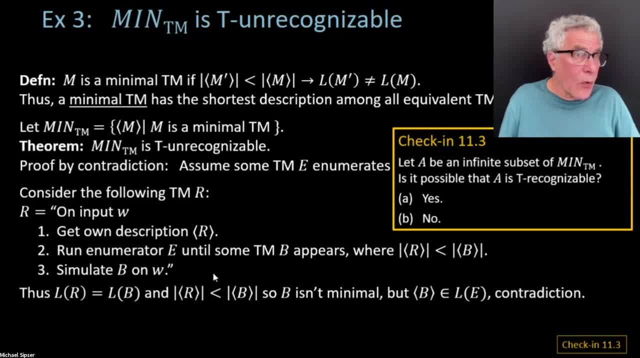 bigger than you appears, And that's all that R needs to do is wait until one that's bigger than R appears- Which will certainly happen eventually if the subset is infinite- And then R simulates that bigger machine and acts the same way. 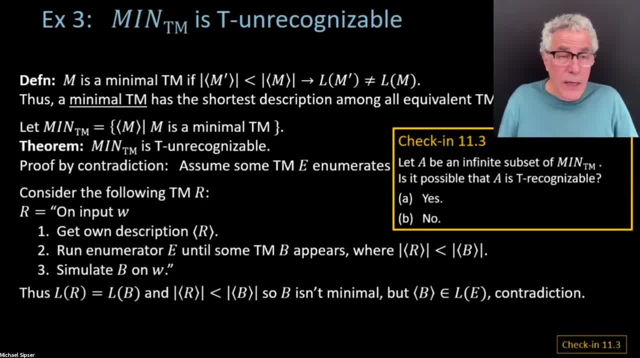 Thereby proving it could not be minimal. So it's exactly the same proof Shows that the answer here is no, And it's a kind of a curiosity. It's not necessarily that easy to construct languages which, not only are they not recognizable, 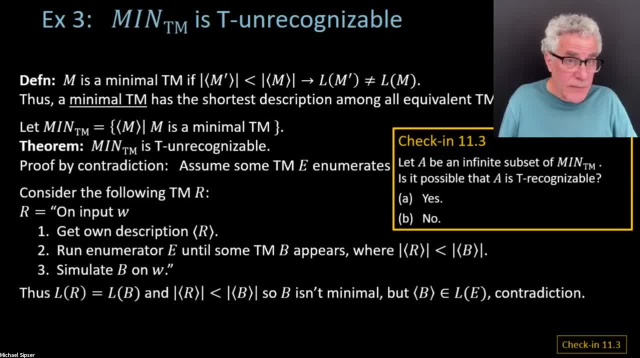 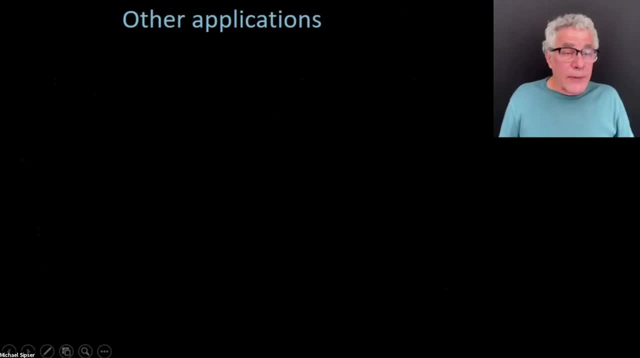 but they have no recognition. OK, They're not recognizable subsets, infinite subsets: Obviously, a finite subset is going to be recognizable because it would be decidable as well. OK, so anyway, let's move on. Some other applications. 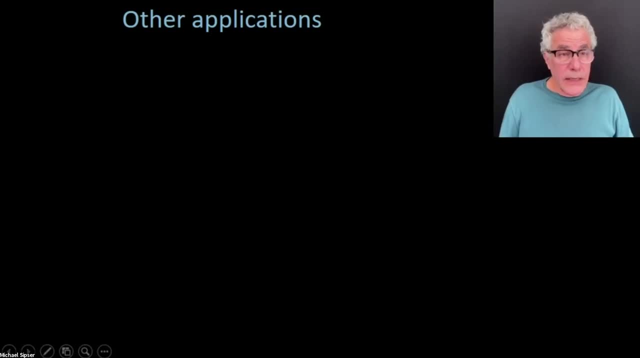 So first, a real world application. So somebody is asking for an example of a language, of a recognizable subset of a non-recognizable language. So starting out with something which is not recognizable, And what can we come up with? a quick. 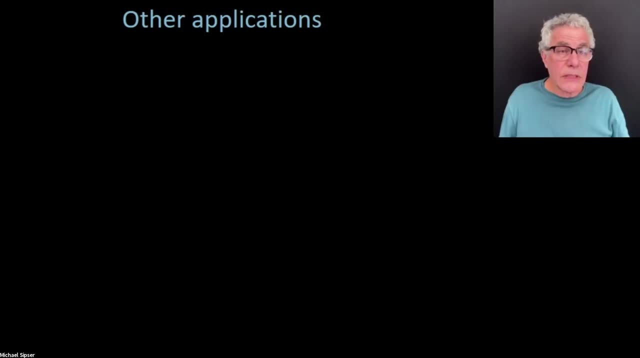 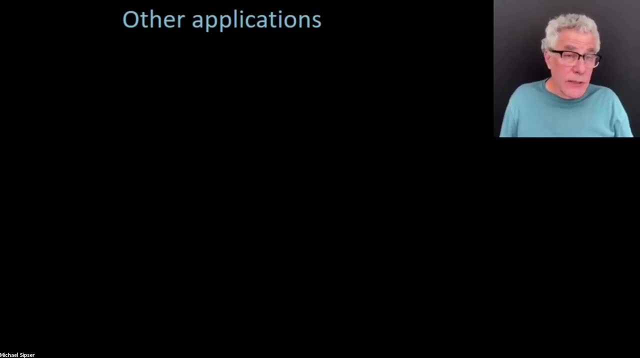 of a non-recognizable language that has a recognizable subset, So I didn't prepare this, but let me see if this helps you. So let's take ATM complement. We already showed that ATM complement is not recognizable. So these are the sets of pairs M and W where. 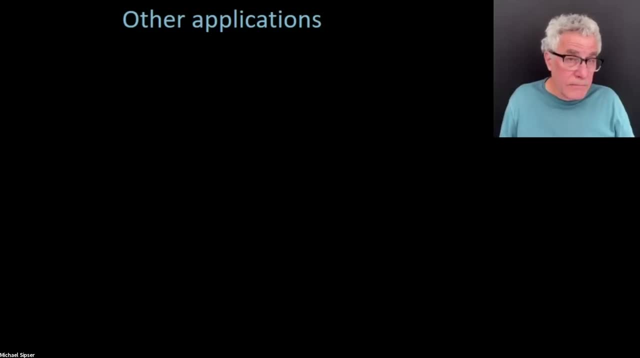 M does not accept W. So if I focus only on those M's which are finite automata, which are a subclass of Turing machines, then I can get the answer for those M's. So for the infinitely many cases where the Turing machine never writes on its tape, I can. 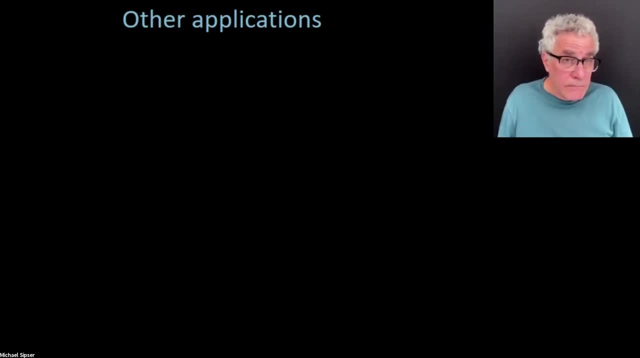 It even becomes decidable. So I don't know if that's helpful, But you can definitely find cases where there are undecidable languages that have decidable subsets, unrecognizable languages that have recognizable infinite subsets. But there is one example where it's not true. 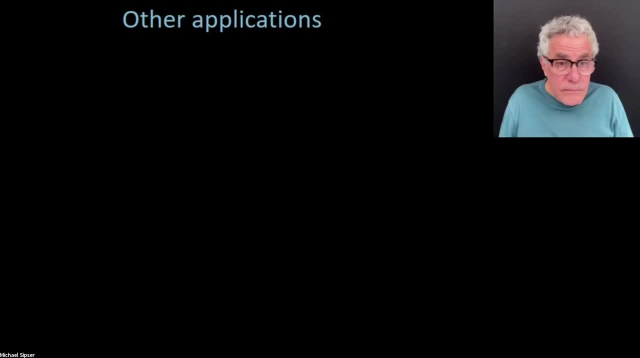 in the previous slide. So that's the one example. OK, a lot of questions coming up here. Yes, I'm seeing some other proposals here. If you take ATM complement and you union it with just all strings of 1s, just one star. 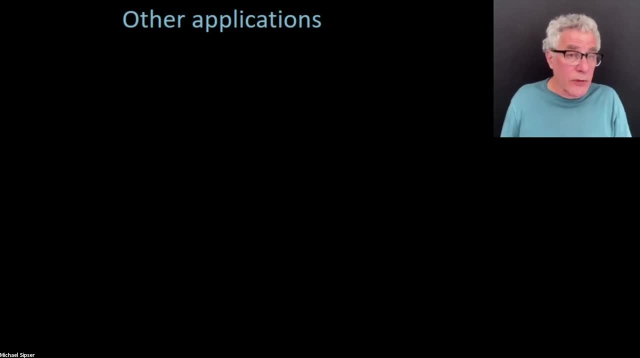 assuming that one star, just strings of 1s, are never going to code for a Turing machine that's still going to be unrecognizable. But then you can just throw away. Throw away all of those, just strings of 1s. 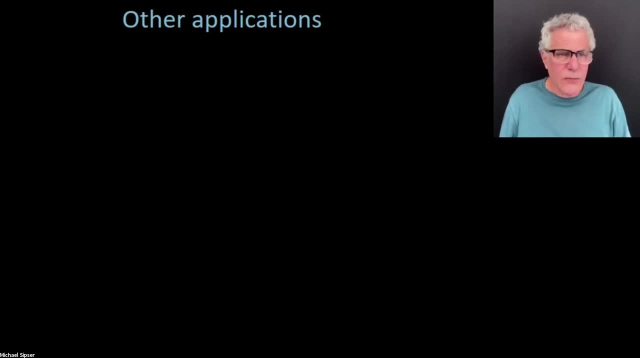 and you're going to get an infinite subset. Oh wait, a minute Still unrecognizable. That's not good. Oh no, yeah, I threw away the wrong stuff. You throw away the descriptions of the Turing machines and you just have the one star strings left. 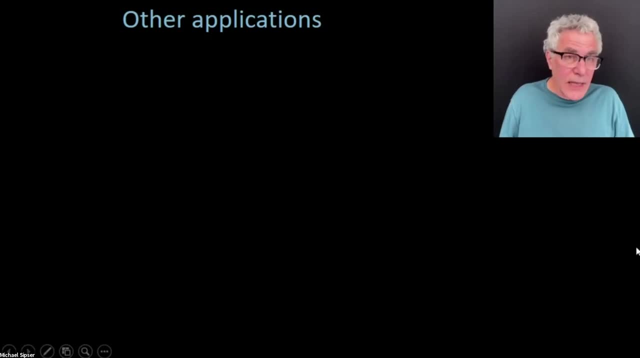 And so that becomes decidable, even regular. Anyway, I think I'm not sure I'm helping you. Let's move on to other applications. So this is kind of a cure, Curious application that actually is in a real world where a machine might. 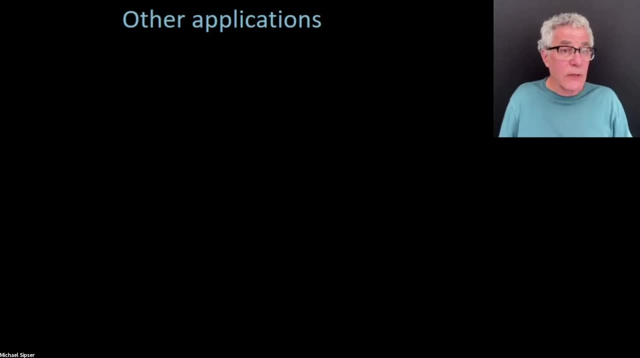 want to get a copy of itself and then do something, perhaps even nefarious, with a copy of its own code, And that would be a computer virus. Computer viruses make copies of themselves and then propagate them through the internet or whatever media you have. You have to use the internet to infect other computers. 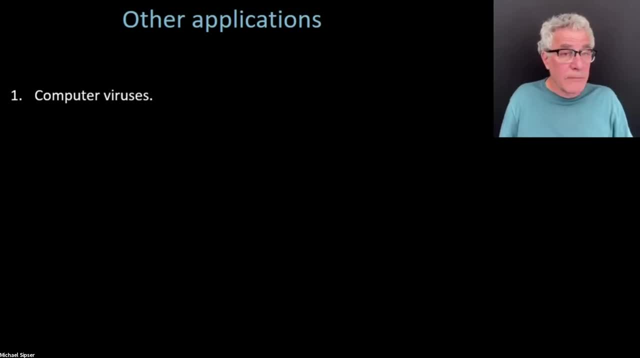 And I'm sure we all know about computer viruses. Well, they need to get copies of themselves in order to do that, to do the infection. How do they do that? Many of them operate in a way where either in a language or in a system where they can make reference to their own code. either by looking at the code, the machine code or whatever, direct access to their own code. There are languages which allow and systems which allow for that, But I'm not an expert on computer viruses. I would be shocked if there are not some other viruses that get access to their own code by using something you know. 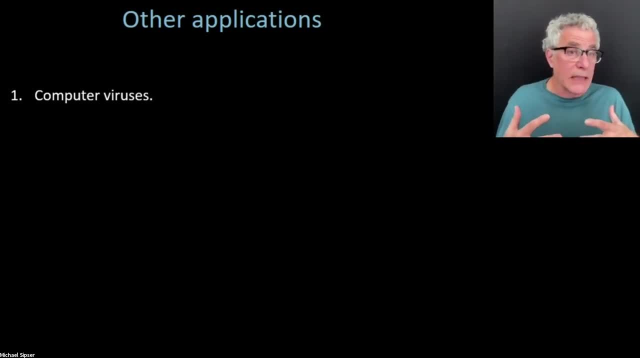 in the same, using basically the method of the recursion theorem. You know I haven't done a systematic study, but I'm sure if you can't access to your own code directly using some operating system mechanism, some primitive, the only other way is basically doing the method that we just 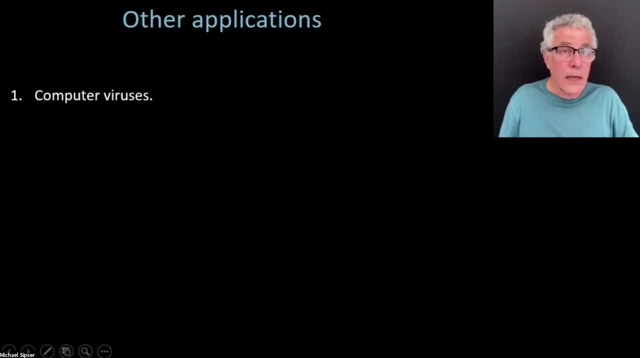 described. Okay, so another application is in a branch of mathematics called mathematical logic, where I imagine that many, Many of you have heard of the work of Gödel from the earlier part of the 20th century, where they show that you can come up, it's possible to demonstrate that there are true mathematical statements, but which? 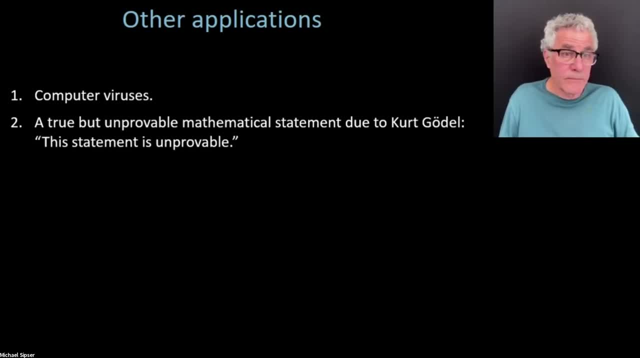 cannot be proven to be true. So proof there might be, something like- maybe even you know, questions of interest to us, you know, like the P versus NP question which we will some at some point look at in a few weeks. 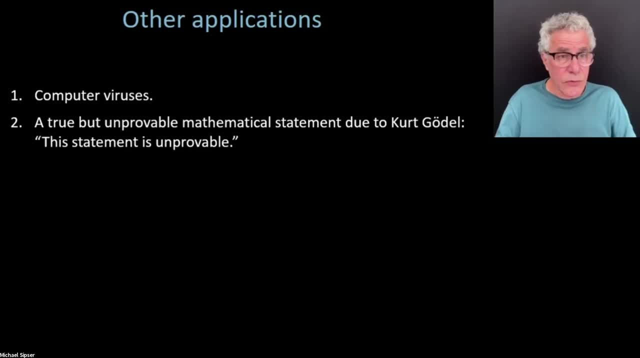 Actually, yeah, maybe two or three, two, two, two weeks from now. There are many unsolved mathematical problems and you know people wonder. You know, maybe there's just no way to prove them one way or the other. 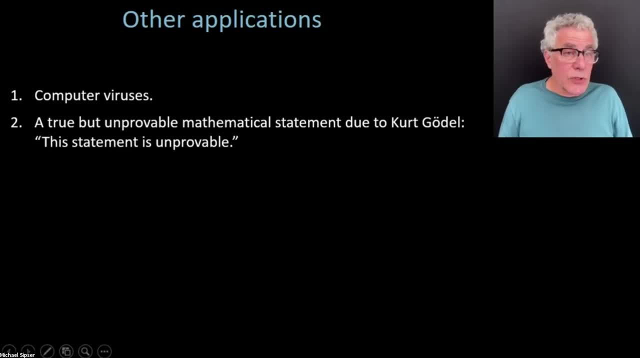 So in the 1930s, when Gödel did his work, he shocked the mathematical community by showing that there are truths, that proof does not work for everything. There may be things that are true that just don't work. You're proven instead. You're proven without question, As the problem is more and more common over the seven centuries and until now. 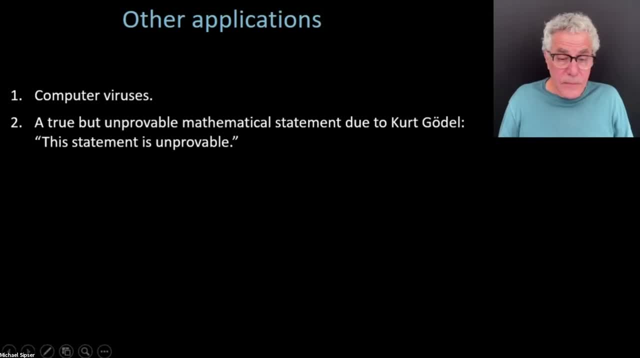 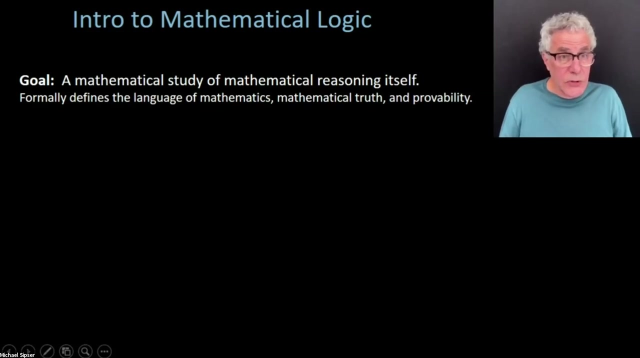 that you cannot prove. Hilbert in particular from Hilbert's 10th problem. he was dismayed by this result because he had earlier believed that anything that was true you could prove. So anyway, let's just see how I'm going to sketch, how we actually go about doing that. 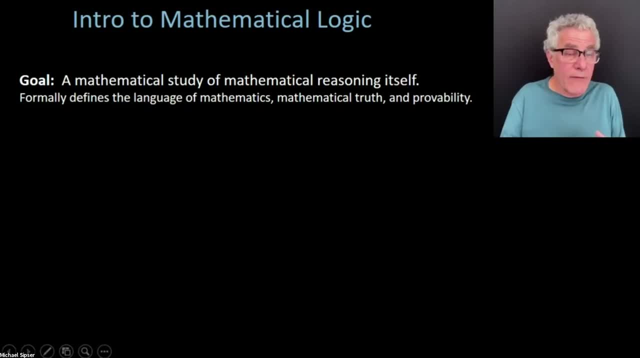 because we now have kind of enough technique to at least give you an idea of how do you demonstrate that there are true but unprovable statements and actually even exhibit one. OK, mathematical logic is the mathematical study of mathematics itself. Gödel's first incompleteness theorem, as we described, 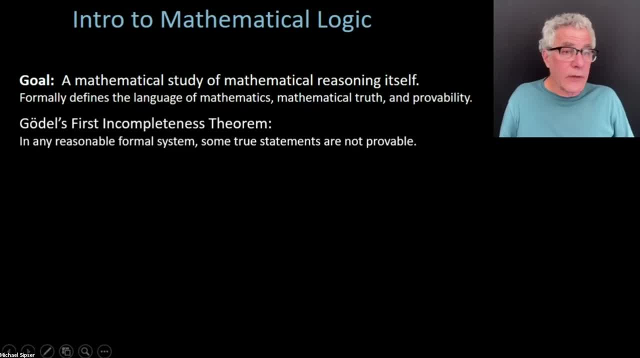 is that in any reasonable formal system of mathematical provability, there are going to be some true statements that are not provable. And in order to sort of get the sketch of the proof- I shouldn't say proof- here We're going to proof sketch. 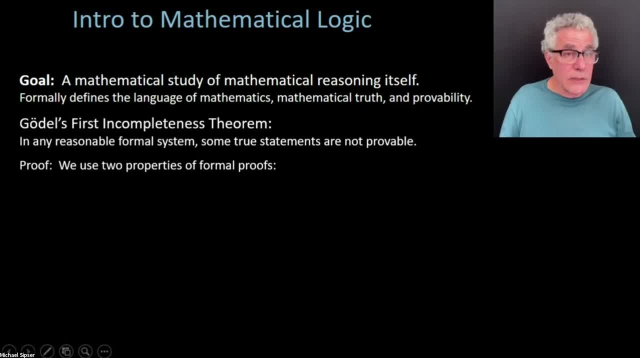 We're going to basically use two properties of formal proof systems. One is that kind of the kind of obvious property that you would expect all provability systems to have is that you can only prove true things. So if something is being proven, it's going to be true. 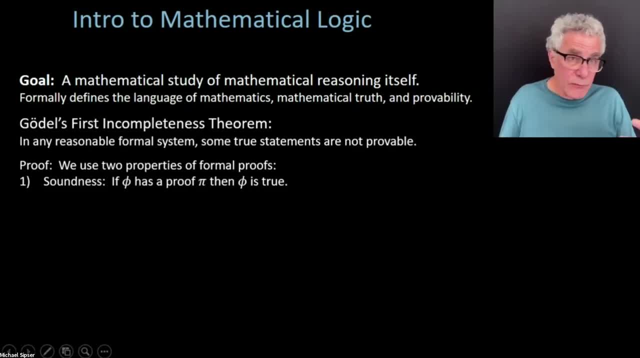 You can't prove anything false. If you can prove false things, your system of provability is bad. And the other thing is that proofs are checkable by machine. So if you write down your system in a formal way and you have this formal notion of proofs, which 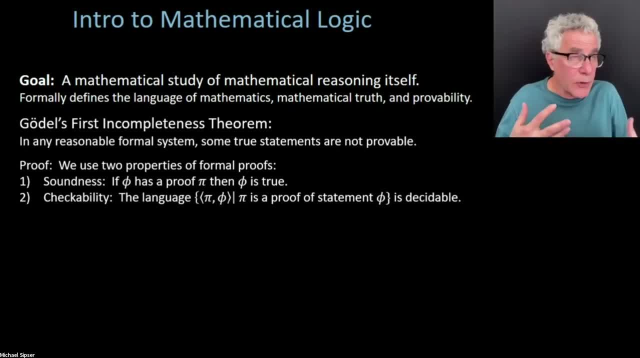 underlies all mathematical reasoning. by the way, This is completely well accepted. Both of these properties are accepted by mathematicians. Then, in principle, you can convert any mathematical proof into a form that you can check it by computer. It might become much longer. 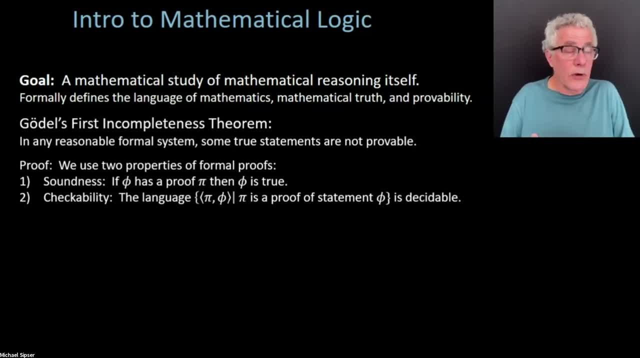 But in principle you can put the proof into a form where a computer could check the proof, And the way we're going to frame that, in the way we've been just talking about things, is that the language of all pairs of proof, comma statement being. 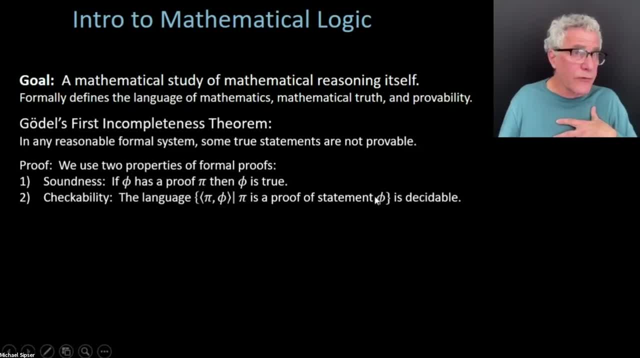 proved so. where the pi is a proof of the statement phi, that's a decidable thing. So you can check by machine whether pi is a valid proof of phi. Your proof checker can say: yes, it's valid, no, not valid. 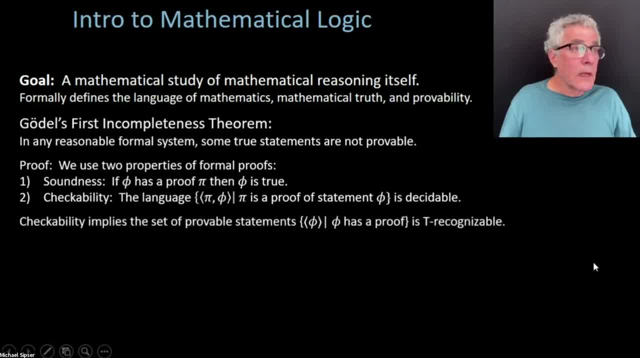 And that's something you can do by algorithm. OK, So those are the two assumptions that we're going to make about our system of proofs, And that's all we're going to need Now, the first conclusion, which is, I think, a good sort of little. 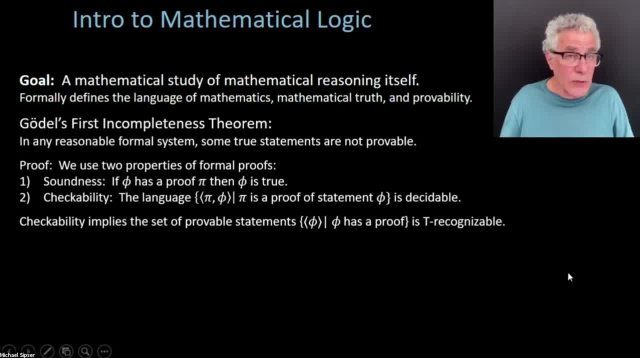 bit exercise on the kind of thinking we've been doing in this course. Number two: checkability implies that the set of provable statements is recognizable. Why, Suppose I give you a statement that has a proof, a provable statement, I'm not saying a true statement necessarily. 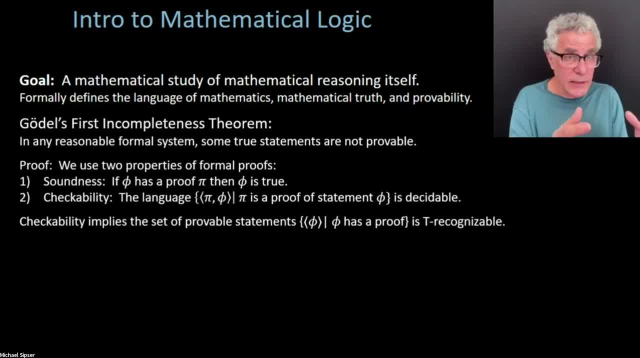 That's going to be perhaps a larger class, perhaps a larger class of proof, But the statements that do have proofs. that's a recognizable language, Because if I give you a statement, your recognizer is going to take that statement and start looking through all possible proofs. 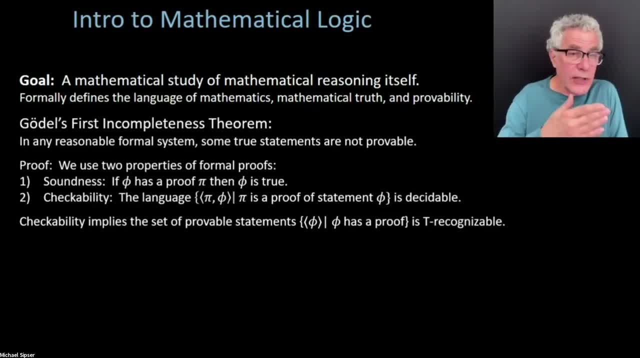 It's going to look at string after string as a candidate proof, one after the next, Some strings, of course, most strings are just going to be junked, But every once in a while, a proof is going to come out. It's going to be a valid string which. 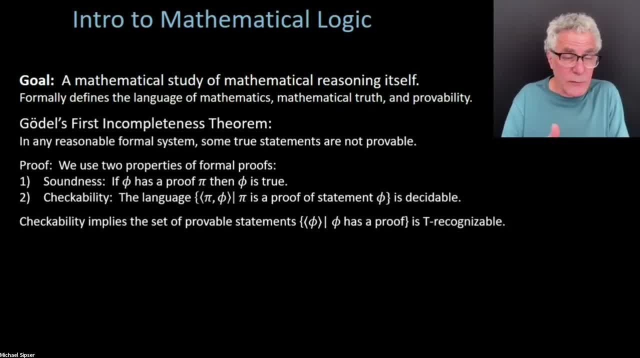 is a valid proof of something, And then you're going to check. oh, let me just see if that's a valid proof And if it does prove the statement that I have in mind, And if it is, then I accept that statement. 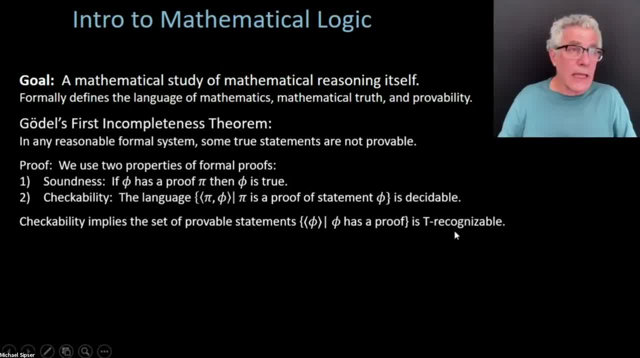 And I go through statement by. you know, the input is a mathematical statement And that's going to be accepted if the machine, by looking through all possible proofs, finds one And then it accepts that statement. So the collection of all statements that have a proof. 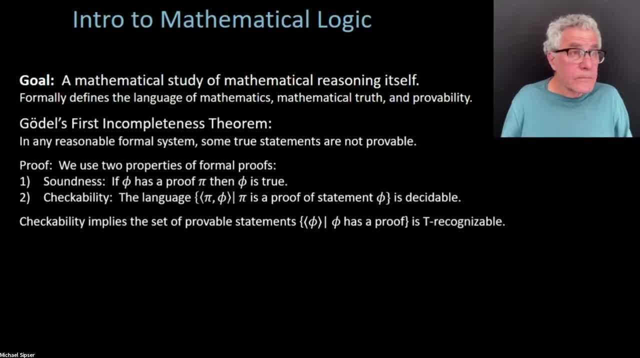 that's recognizable. So, similarly, if you take statements of the form M and W is in the complement of ATM, so M doesn't accept W. If you take all statements of that form where M doesn't accept, so M doesn't accept W, or MW is in the complement. 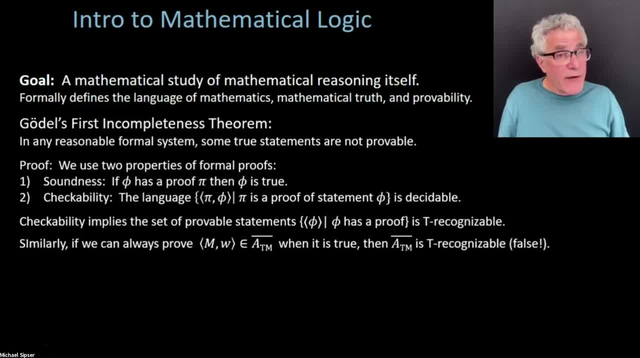 of ATM. some of those statements may have proofs in your system. Some of them may not have proofs. If all of them had proofs, if you can prove every statement of this form when it happens to be true, obviously you can't prove the ones that are not true. 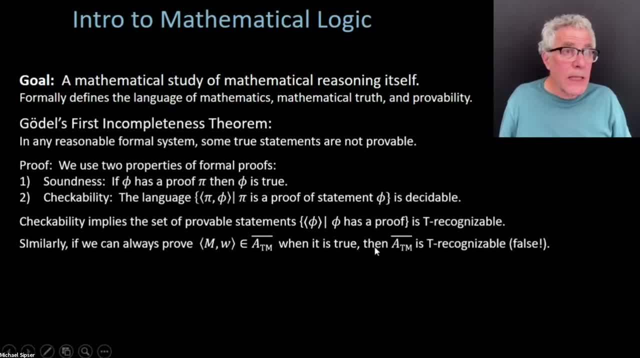 But if you can prove all the true statements of this kind, then ATM complement would be Turing recognizable Because you can go through, You can, just You can prove your statement for the same reason as above. But we know that that's false. 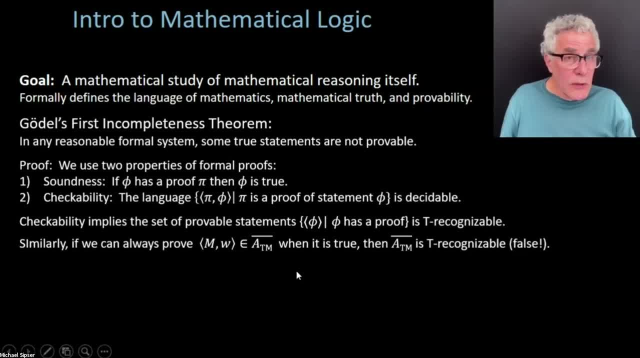 So there must be some statement of this kind which is true but does not have a proof, Because otherwise ATM complement would be recognizable. So we've actually done the first half of Gödel's incompleteness theorem, The second half, which we're going to unfortunately not have time to finish, 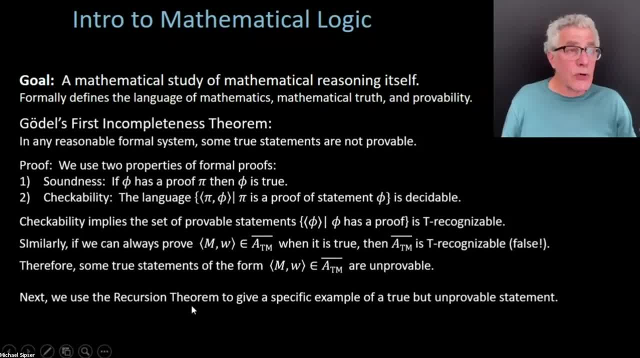 finish- but let me just give you the outline- is that we can use the recursion theorem to give a specific See, what we showed here is that there is some statement of this form which is unprovable, which is true, but unprovable It doesn't exhibit a particular one. Now the 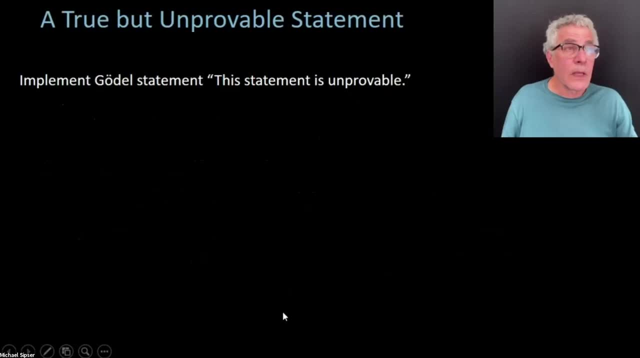 recursion theorem allows you to give a particular one. It basically implements the so-called Gödel statement or Gödel sentence that says this statement is unprovable. You can formalize that precisely and then that statement becomes true but unprovable. Let's just say: 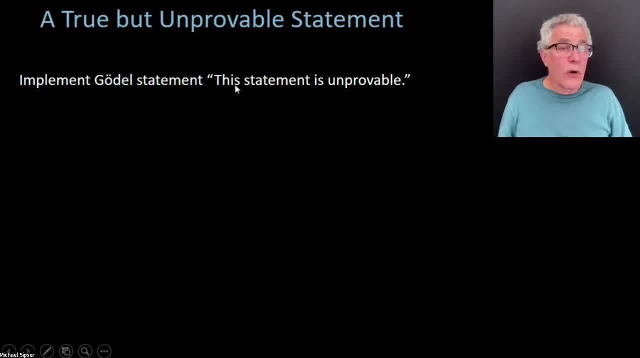 why? that is Because if the statement were false- suppose the statement were false- then it would be provable, Because the statement is unprovable. The truth says it's not provable, But if the statement were provable, then it had to. 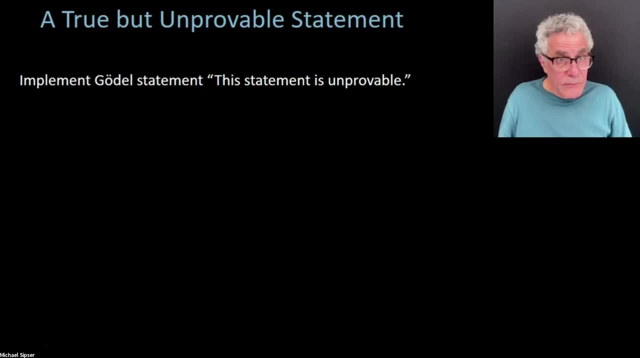 be true, which would mean it would be unprovable. The only viable outcome here is that the statement is unprovable and therefore that it's true that it's unprovable, so that this is a true statement, but then it has no proof. Let me not go through it because again we're going. 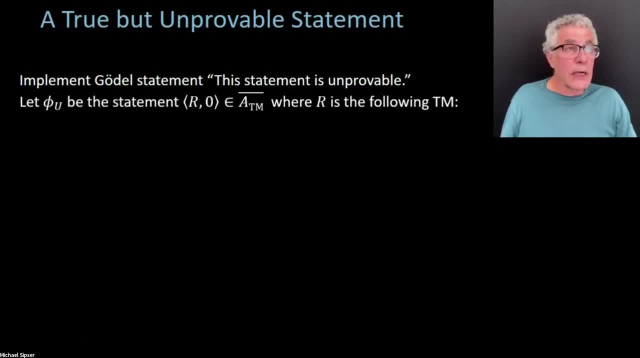 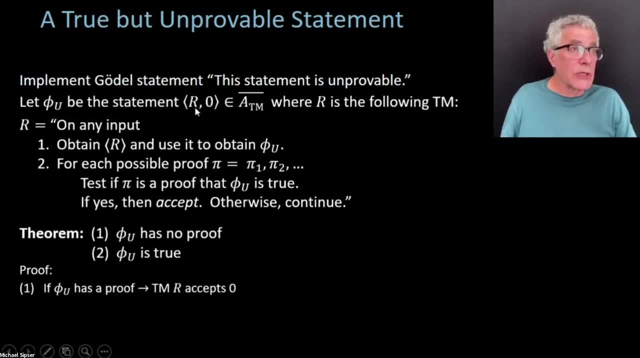 to go through it. I unfortunately ran short on time. But you can implement this using the recursion theorem to make a particular machine r where you cannot prove that r does not accept, say, some string 0. So you can find a particular r using the recursion theorem where it's impossible to prove that. 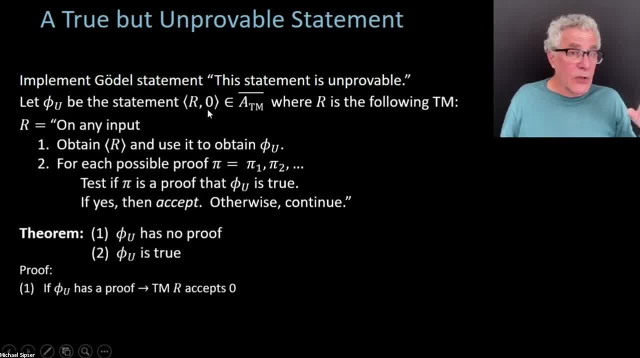 r doesn't accept 0. Even though, by construction, r does not accept 0. So it's a little bit slippery there, because you have to understand what we mean by proof within the formal system versus our external form of reasoning. but taking us a little, 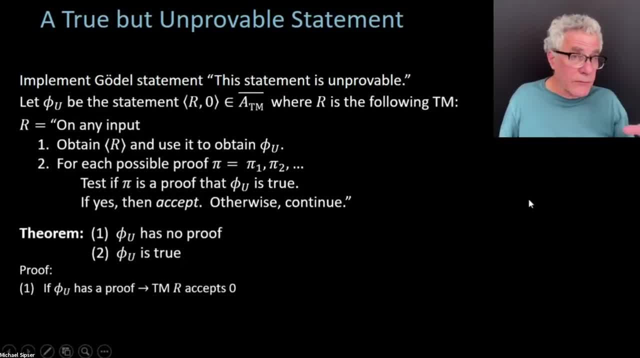 bit far afield. So, for those of you who care, I hope this little digression was interesting. As I mentioned at the beginning, for those of you who don't care, you don't have to worry about it. It's not going to be on the midterm or on the final exam. 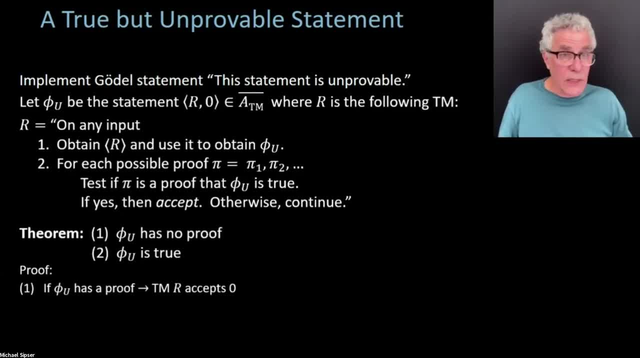 You're not going to be responsible for this last you know four-year period. It's not going to be on the midterm or on the final exam, It's going to last you know five minutes or so of the lecture. But I thought it's kind of an interesting application of the recursion theorem to a. 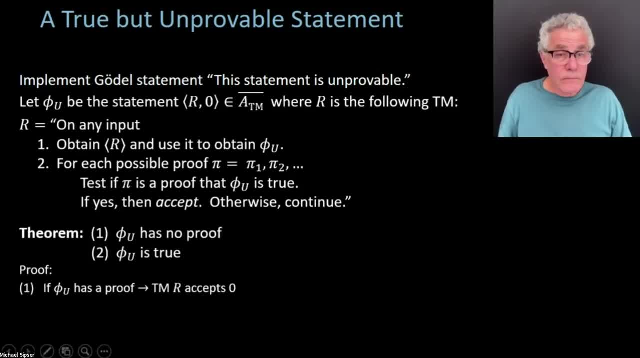 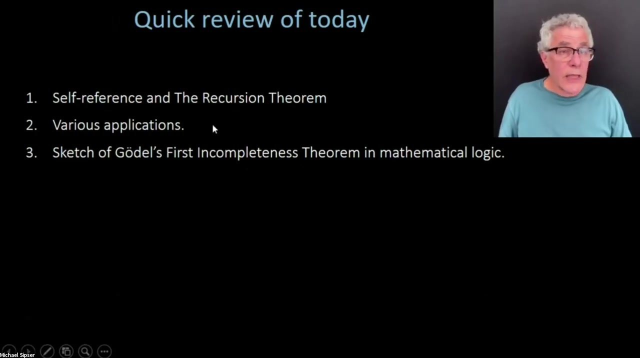 problem outside of computer science in mathematical logic. OK, So here's the entire reasoning. here Again, I invite you to look at that on the slide that I've posted if you're curious. So anyway, quick review of today. We went through the self-reference and the recursion theorem. 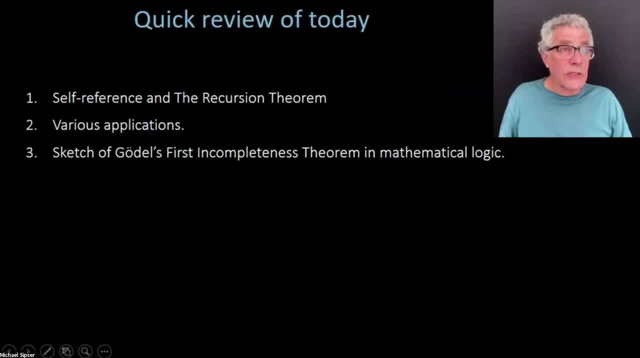 We gave a few applications And we did a sketch of Gödel's first incompleteness theorem in mathematical logic. OK, So that's all I'm going to have for you today. We're out of time And I will take any questions. 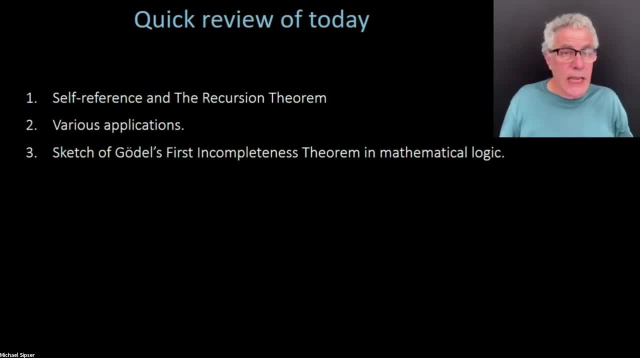 So, getting back to the min Turing machine example, somebody is asking: how do I know there's a Turing machine that's longer than the machine R that I'm building? Well, there are infinitely many machines In minTM Or in the infinite subset of minTM. 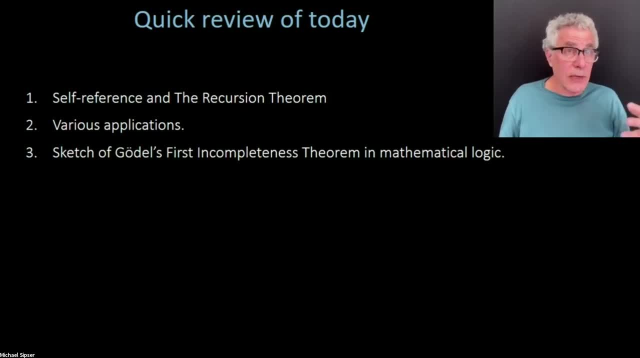 So eventually, one of them is going to have to be longer than the machine that I'm constructing, Because that's a machine of some very specific size, And so eventually there's going to have to be one that's bigger. that shows up. 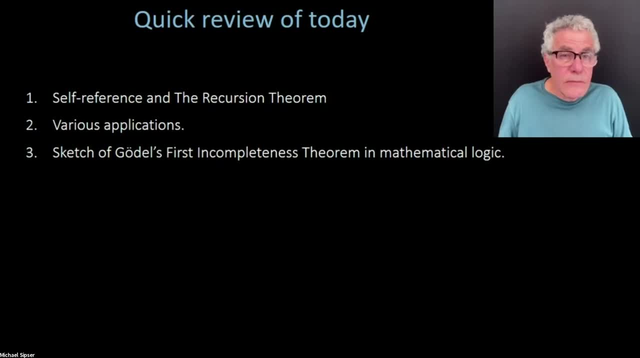 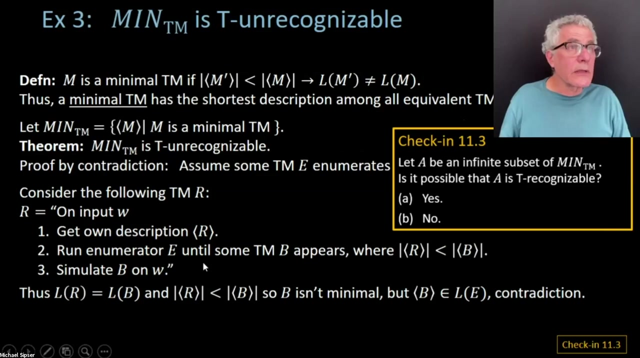 So this may be a similar question Given Now. another similar question is about how big is R, And does R the size of R in that previous thing here? I don't know if we want to go through this, but OK, let's quickly look at it. 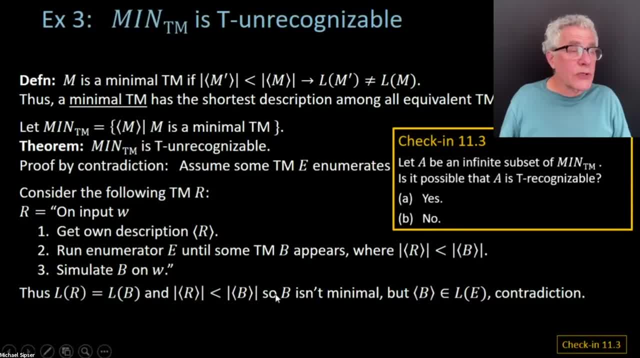 This machine R has a fixed, predetermined size. Its size does not depend on B. I mean it depends on E, because it's going to be simulating E, But E might be a norm. It's going to be producing very, very long strings. 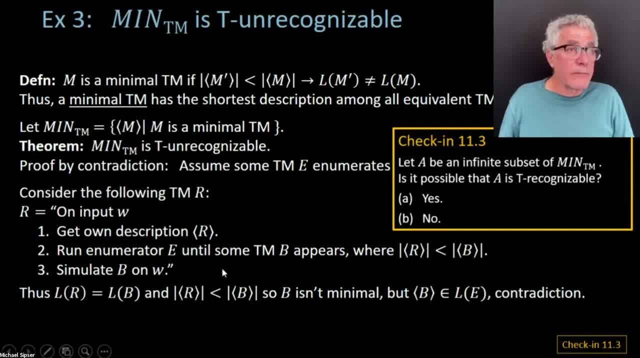 Eventually it will. So E is fixed and then R's size is fixed. So eventually R will find a machine that's bigger than it is. But let's look at the right. So this is a good question. I was wondering if I would get questions of this kind. 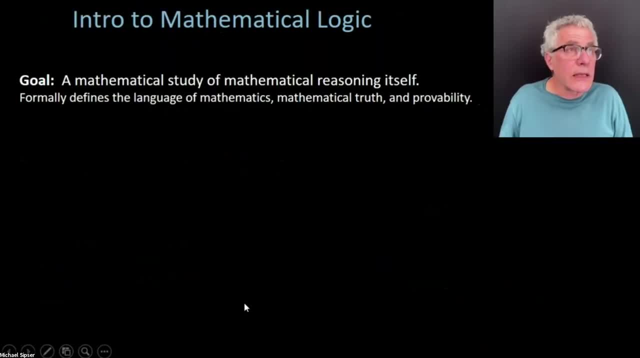 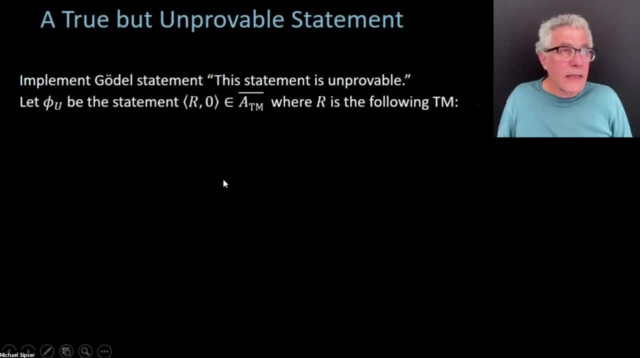 This is getting back to the question. I'm in logic here at the end, Yes, because I said this statement here is unprovable. But in a sense I proved it, Because how do I know it's true And I gave you an argument for it. 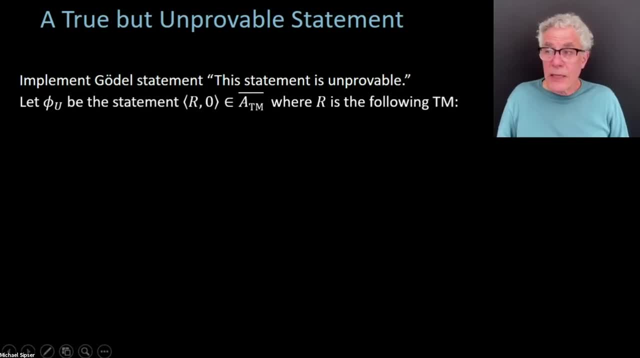 And so you have to differentiate between the reasoning that we're providing and the formal system that we're reasoning about. And the formal system that we're reasoning about is not capable of proving this, But we're outside that formal system so that we can reason about the formal system. 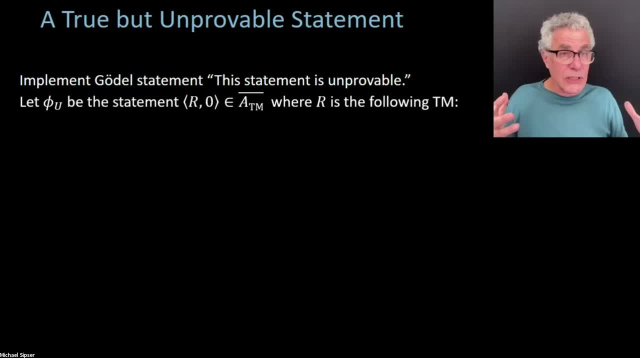 I know it's a little bit perverse-seeming and mathematical logic is a little tricky because it has to deal with those kinds of issues. But this is arguing within any particular formal system of provability. this is going to be true, But you know. 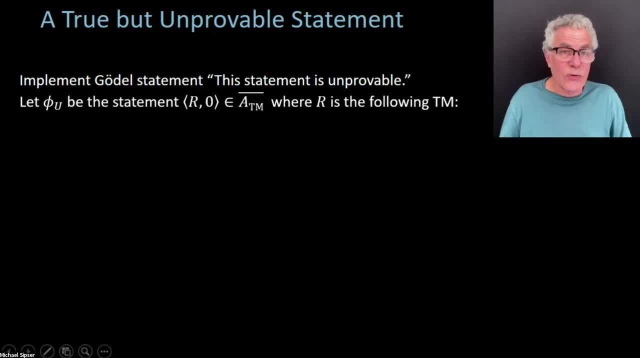 So that's kind of an approximation to our own thought process. So it's slippery, I agree. So a quick question here: Would Gödel's theorem still hold in formal systems where we don't require that proofs of statements are decidable? So I'm not saying that the proofs are decidable. 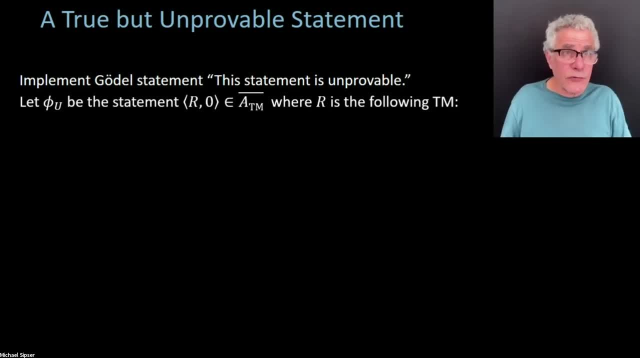 Proofs are checkable, So you can test whether a proof is applicable. If you can't test whether a proof is a proof, I don't know if any people have studied that situation, So that's a little bit of a trickier case. 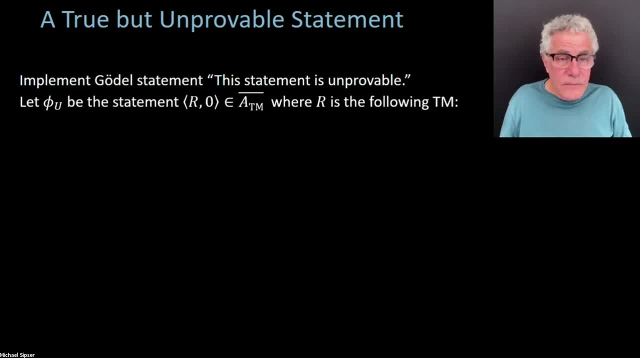 I'm not sure what to say about that. Can I give an example of two equivalent Turing machines where one has a shorter description than the other. How do we define the length of the description? Well, We never really precisely defined our encoding system, but whatever encoding system you want, 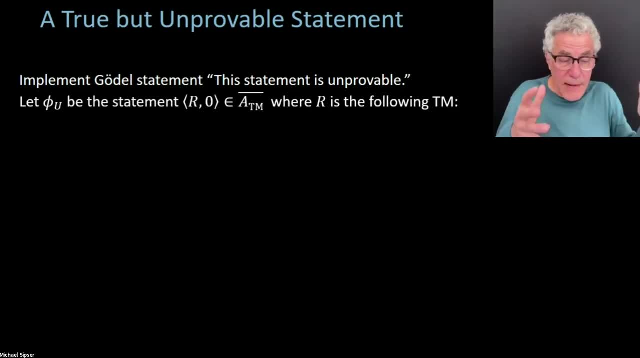 to use is going to represent Turing machines as strings, and those strings are going to have a length, And so it doesn't really matter which encoding system you're going to use, because the statement is going to be true in any of them. We could go through the exercise of defining a particular encoding system.